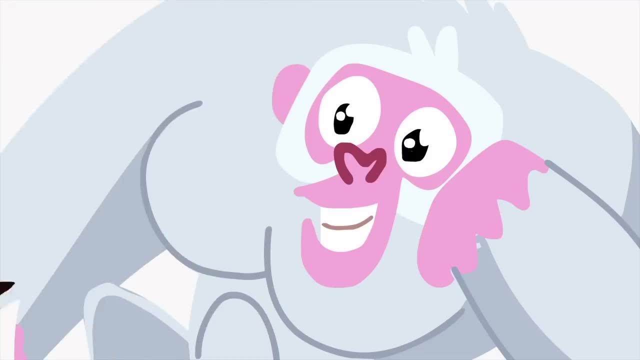 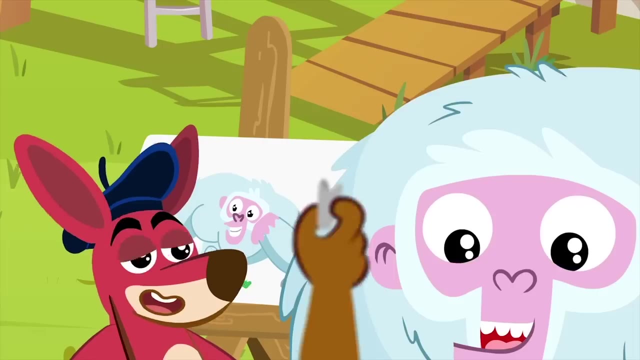 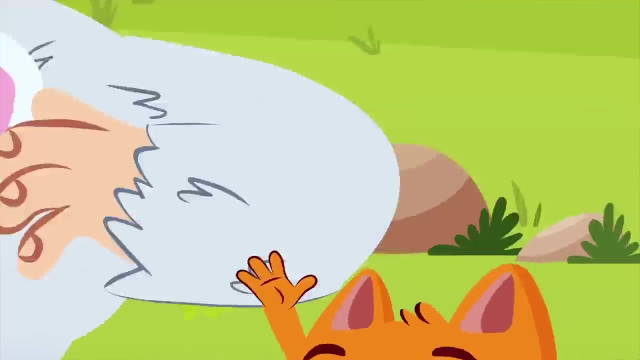 This is great. Come on, Catty, Let's find the others and tell them: Look at Catty's tooth. What do you think the tooth fairy will bring her? It's pretty cool, right? Wait what? Our tooth has been stolen. 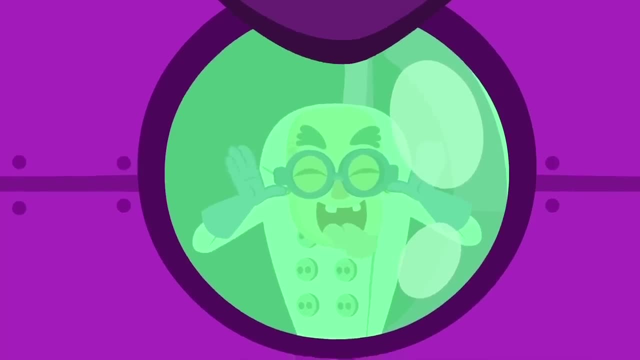 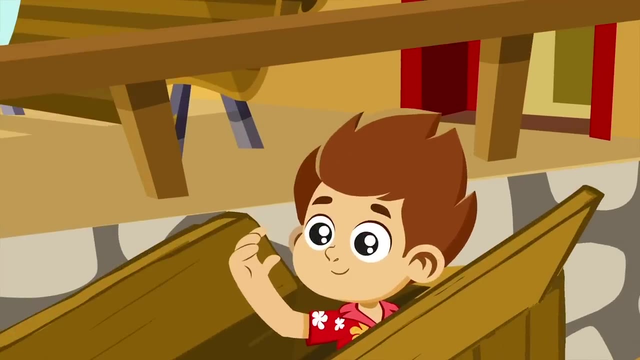 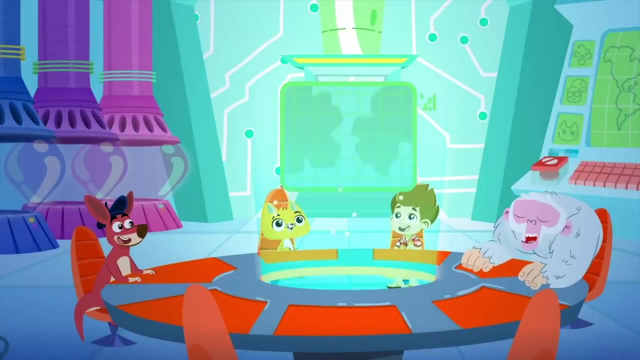 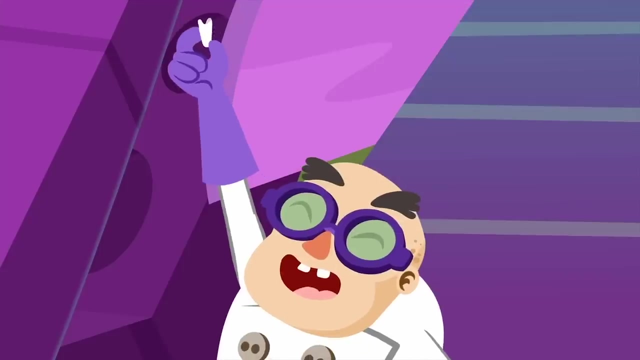 Oh, of course This is Dr Spooky's work. Don't worry, Catty, We'll get what's ours. Kids, Tell us where the tooth is. Come on, There it is. We have to go and retrieve it at Dr Spooky's base. 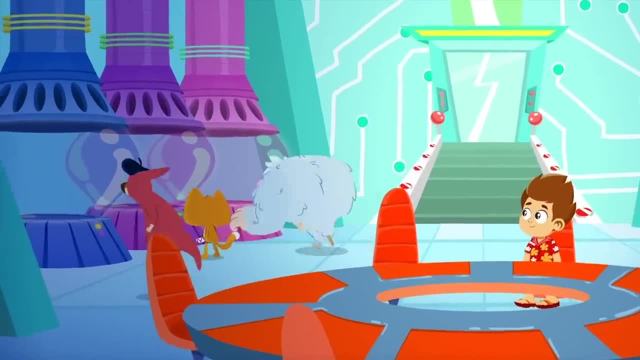 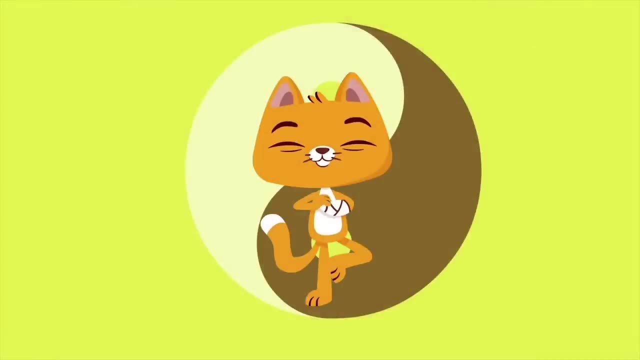 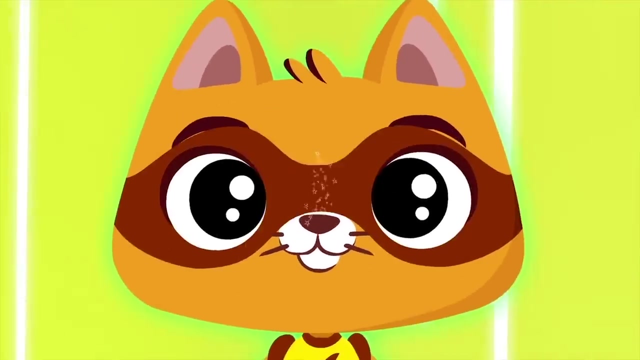 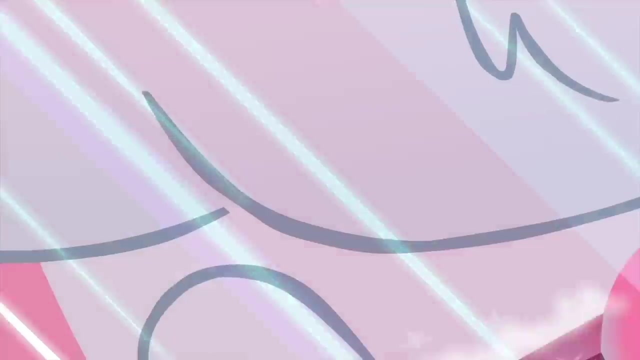 Look at that face. Look, oh, look, at all that. that's my tool. Oh my, that's my tooth. You know, it doesn't make a difference. I've got another one. Peek-a-boo, Go on, I've got another one. 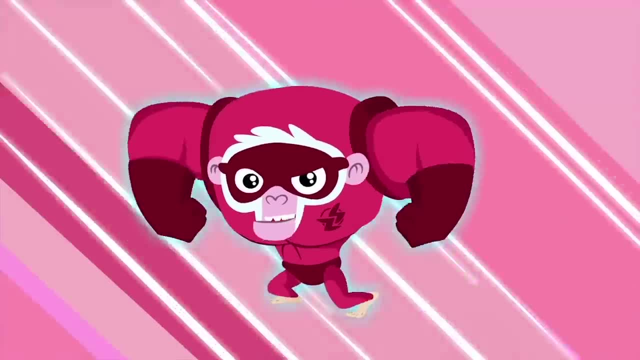 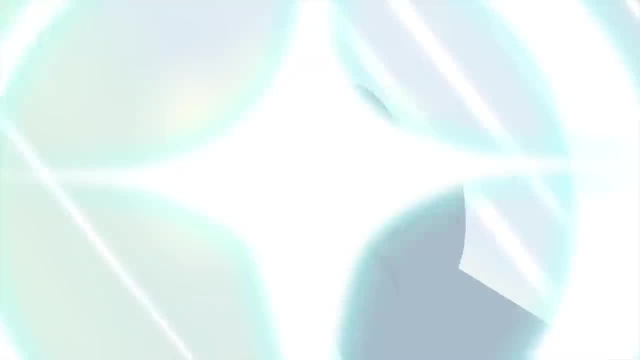 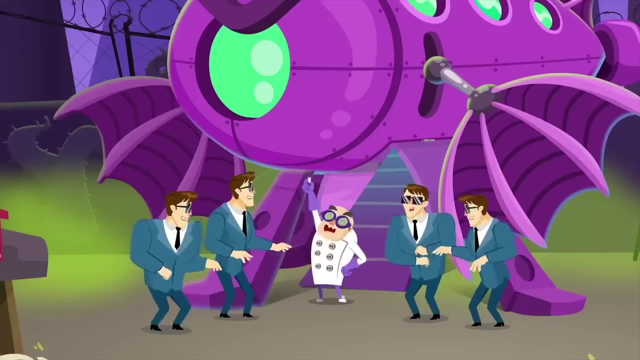 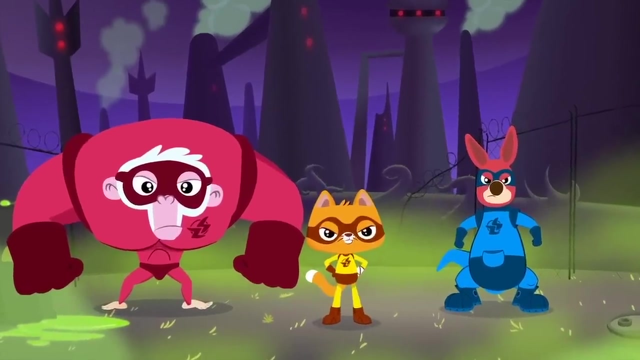 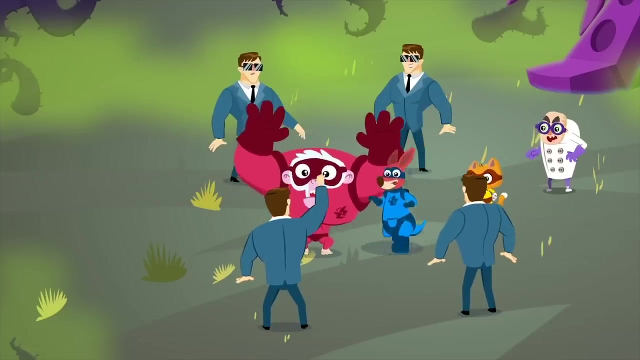 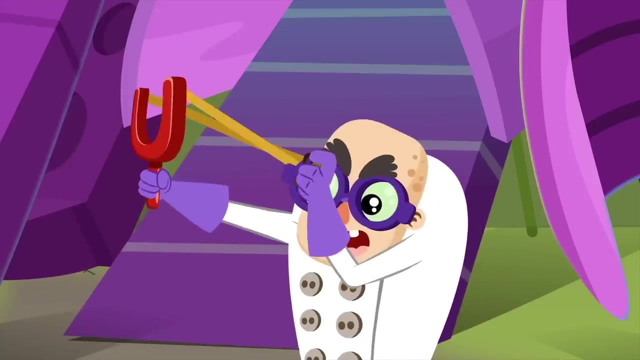 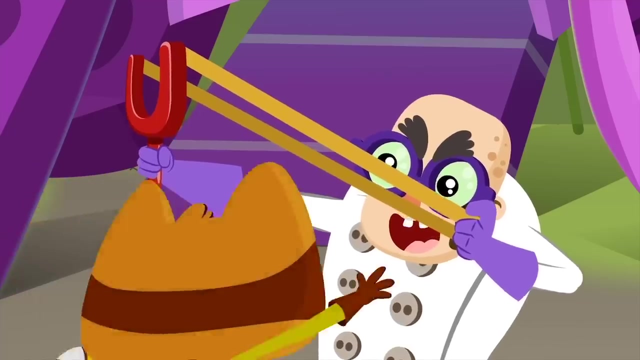 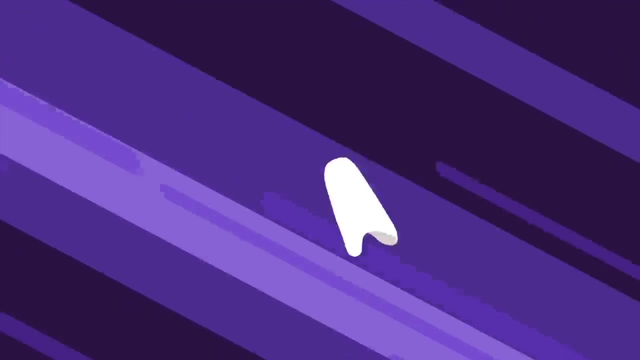 hydrogen, hydrogen, hydrogen, hydrogen. Hmm, here you are, And here is the super zoo team. You better give them their tooth back Now. let's get it back. Stop playing, we want that tooth Now. Be careful. Oh no, How selfish you are Spooky. 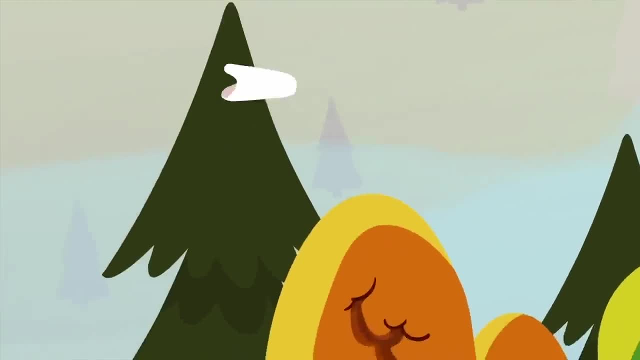 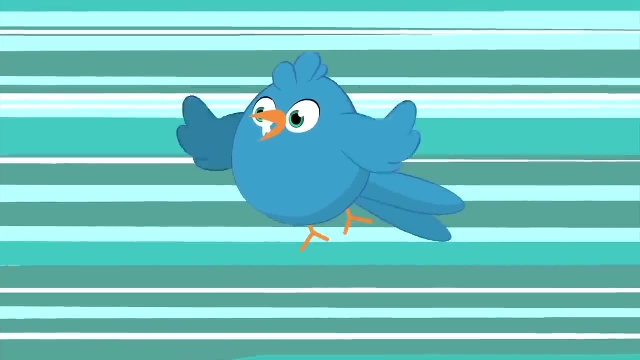 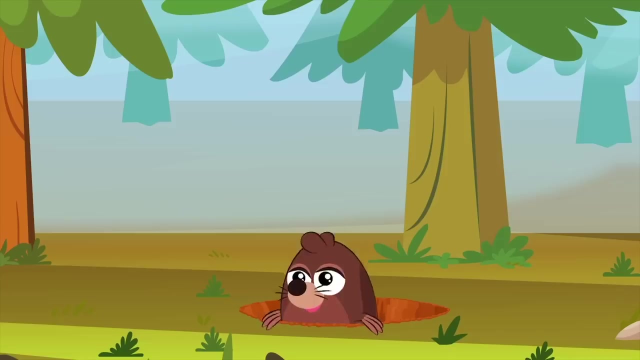 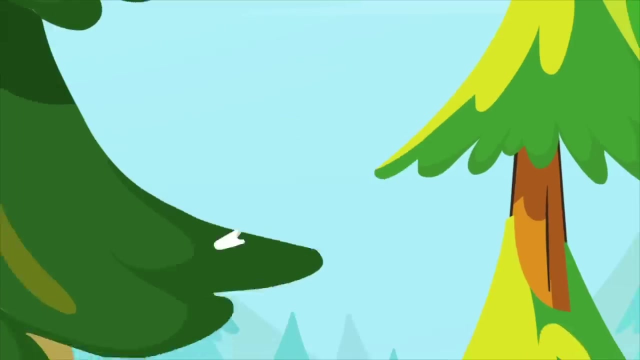 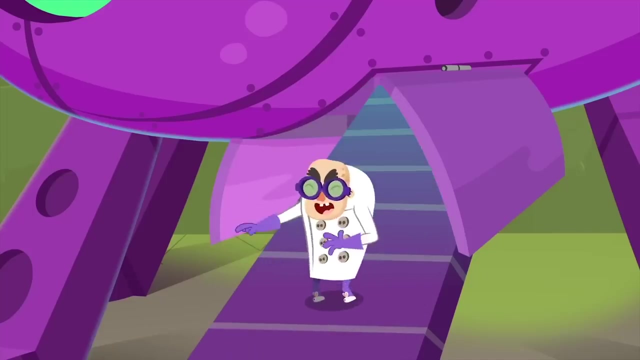 Uh-oh, that tooth really liked to travel. Sorry, Mr Bird, Sorry little bees, Oops, sorry too dear trees, Sorry, Mr Mole. Oh really, This tooth has definitely gone very far. You are so mean, Dr Spooky. 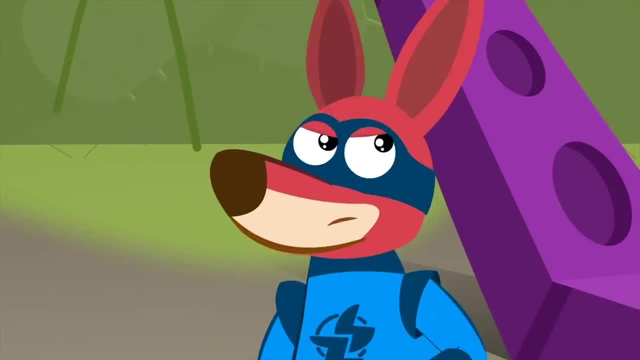 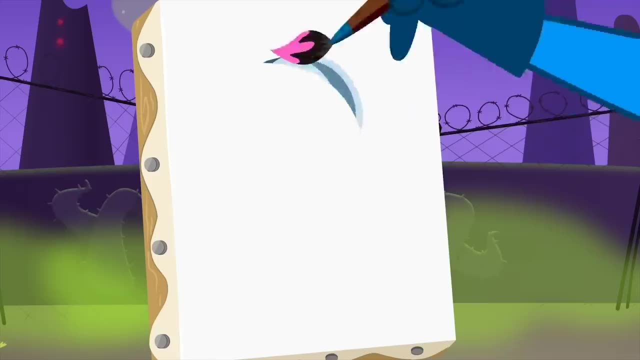 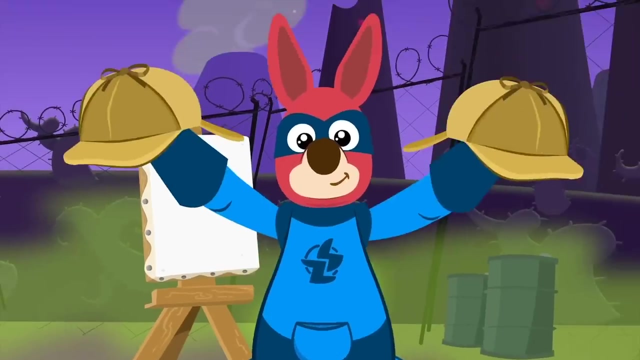 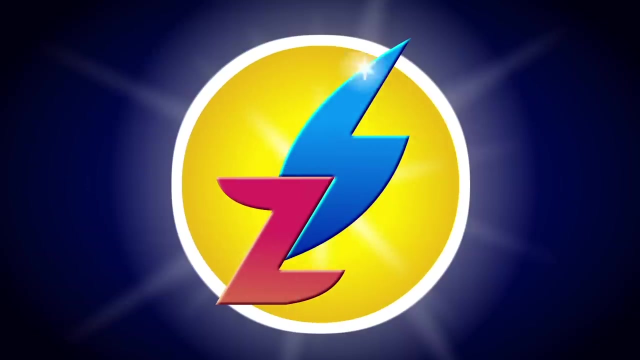 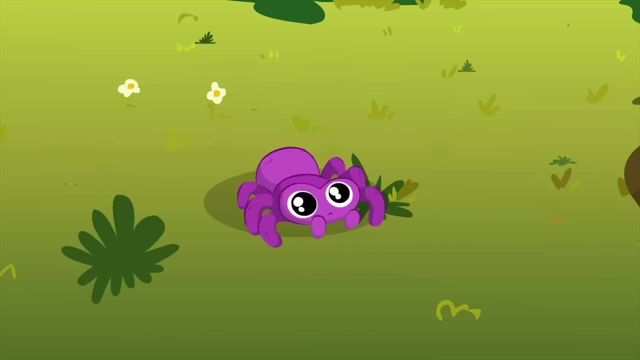 I don't think we can get it back. What Kangoo has an idea? Good idea. Kangoo, With those magnifying glasses, We will miss a single detail. Full detective- look, We will find the tooth. Let's do it. It seems like they haven't seen anything around here. 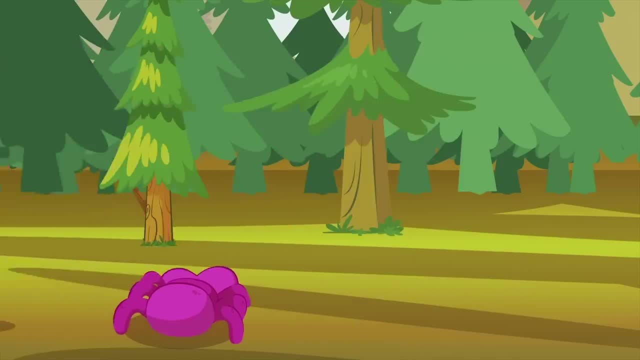 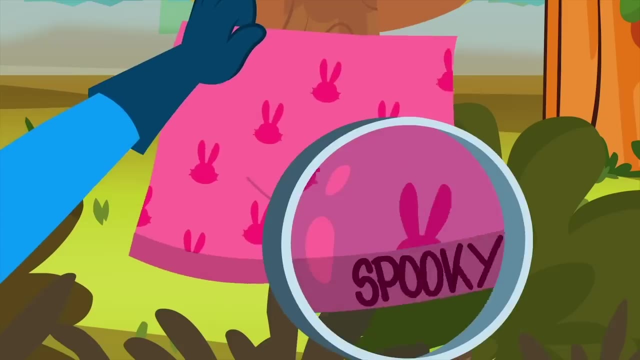 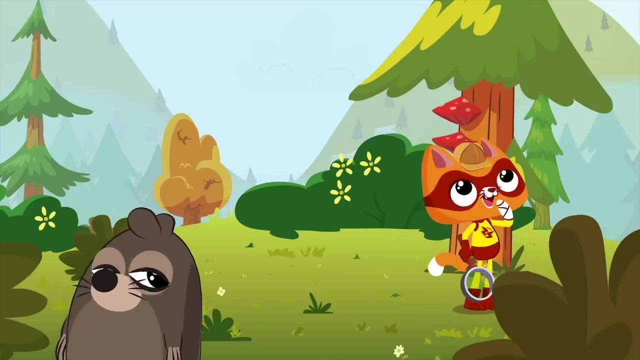 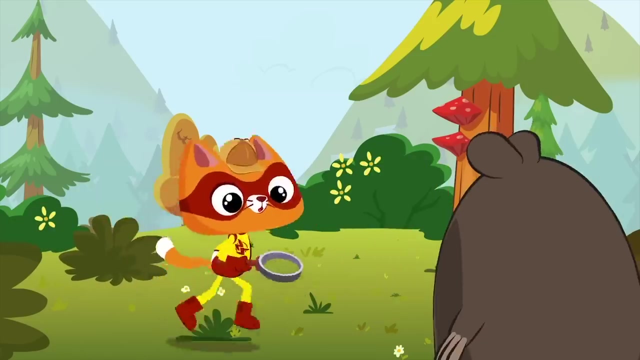 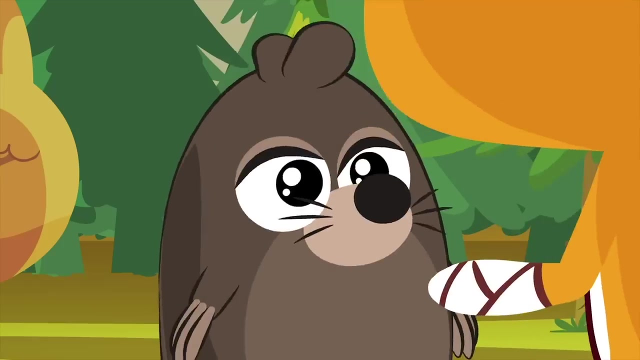 Let's see if Kangoo has had any luck. Oof, Looks like Spooky loves to throw things around. Oh wait, Maybe that mole knows something about the tooth. Hey, Mr Mole, Make it easy for us. It seems that someone has gone to the dentist. 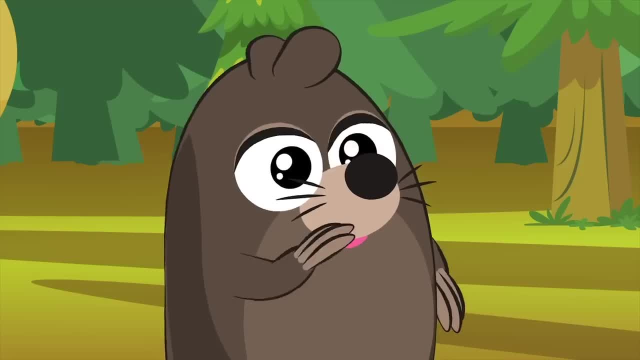 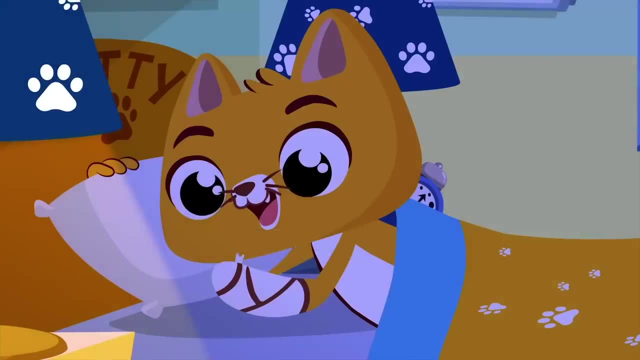 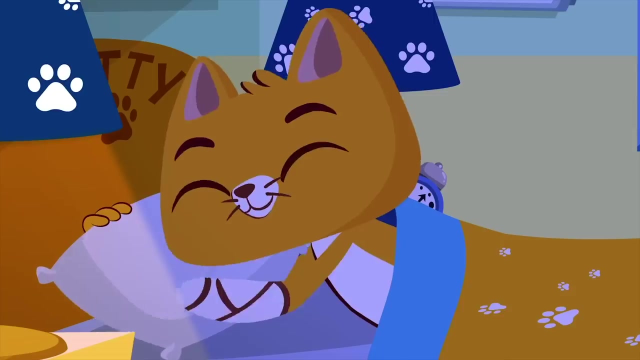 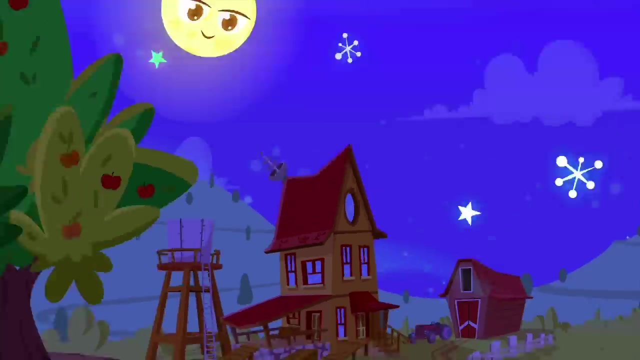 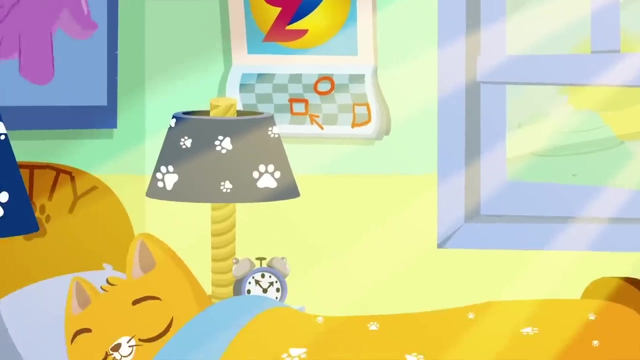 Thank you, Mr Mole. That's right, Catty, For the tooth fairy to bring you a gift. You have to leave it to me, You have to leave it to me, Leave it under the pillow. And now sweet dreams. Good morning, Catty. look under your pillow. 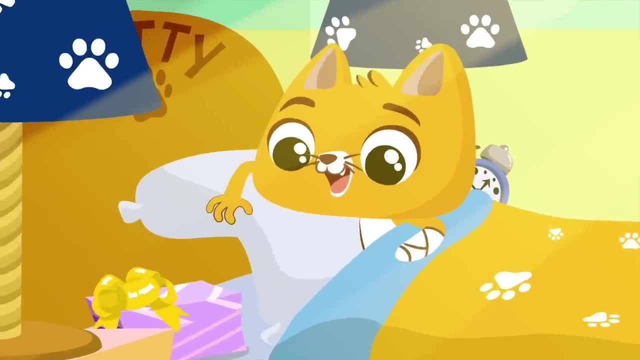 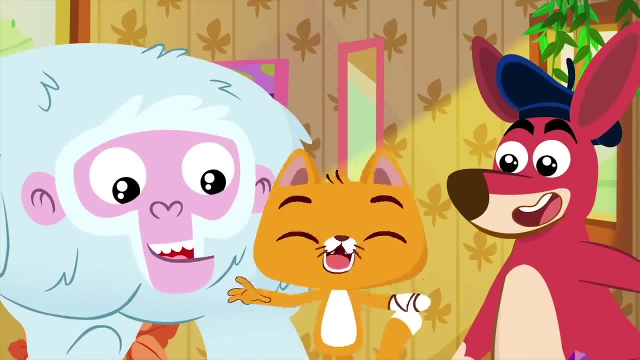 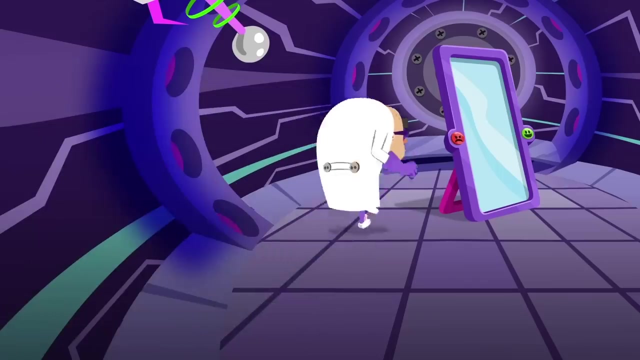 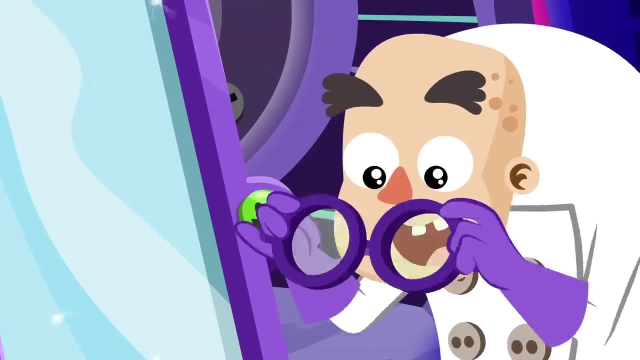 I think someone came tonight. Oh, there it is. Hey, the tooth fairy came. Oh, Super Sweet. Team always wins. What is Spooky doing? What a weird mirror. It's got a bad and angry button And a good and happy button. 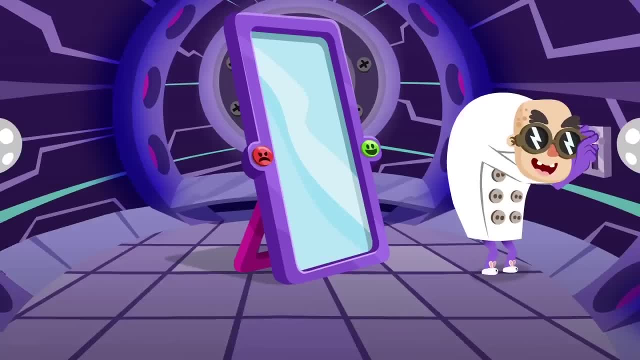 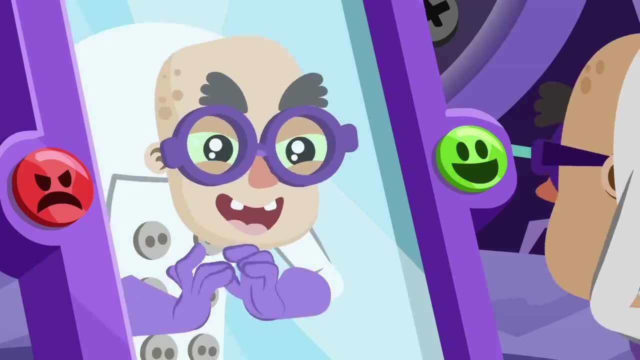 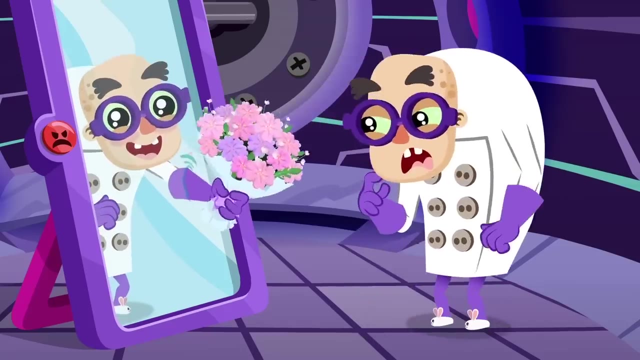 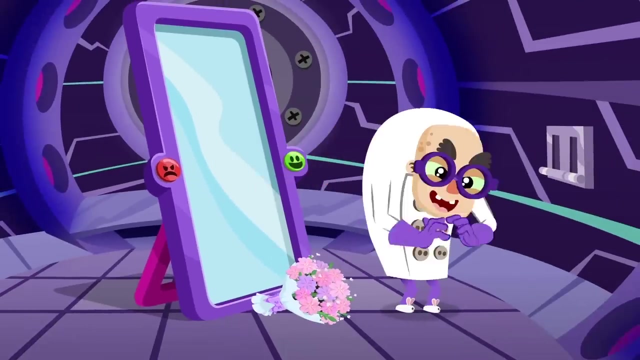 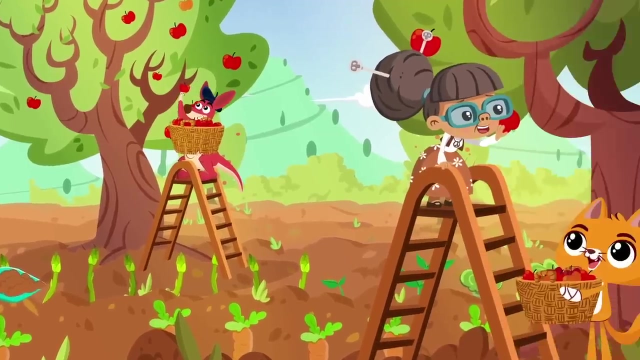 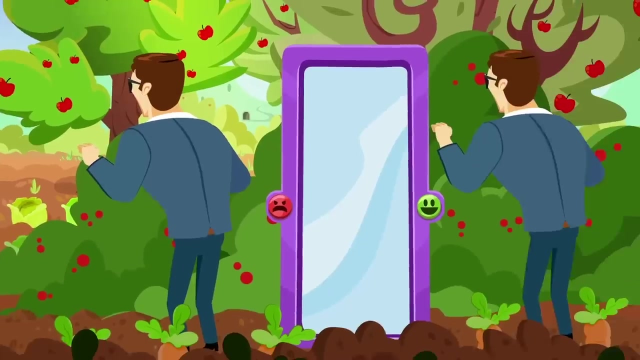 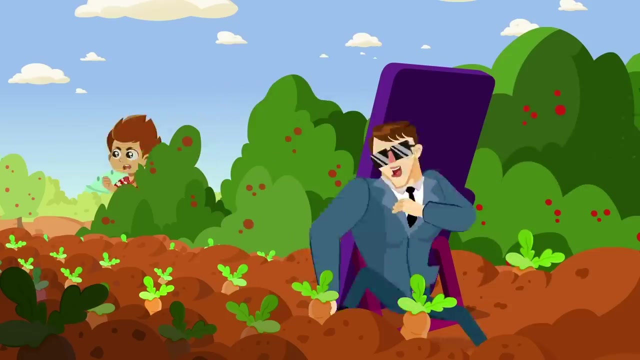 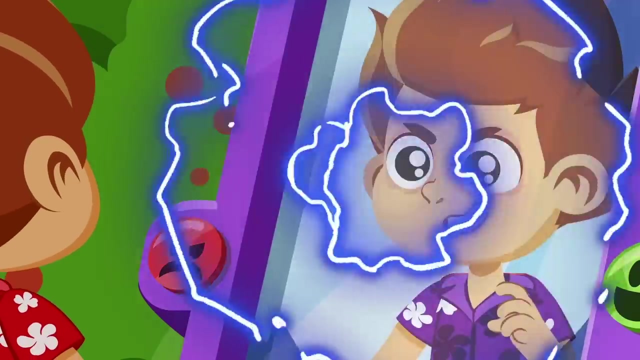 And now what, What, What, What? It's a magic mirror. Oh, I really like the flowers. What a great day to take care of the environment, as always. What's the mirror doing there? Um, kids, I don't think it's. 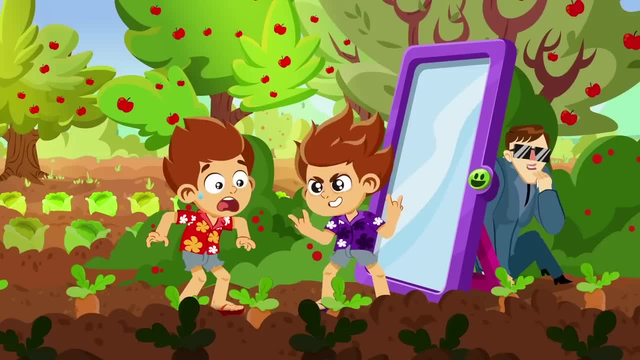 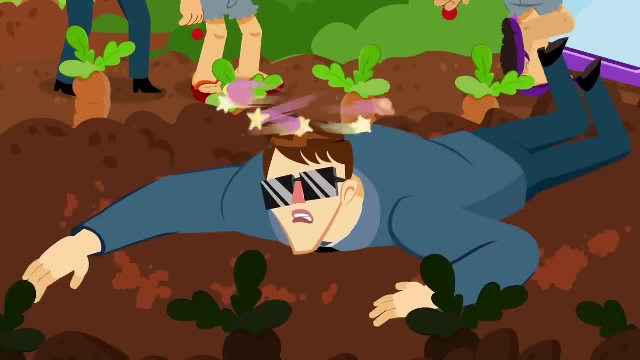 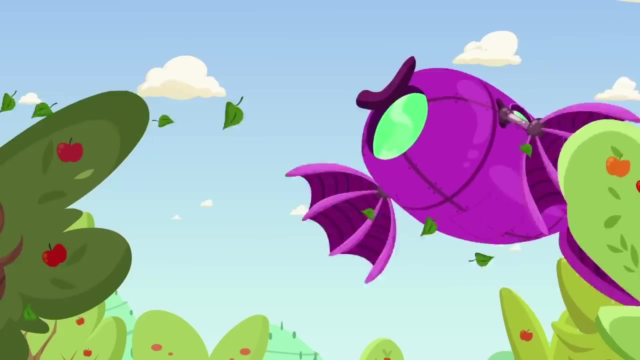 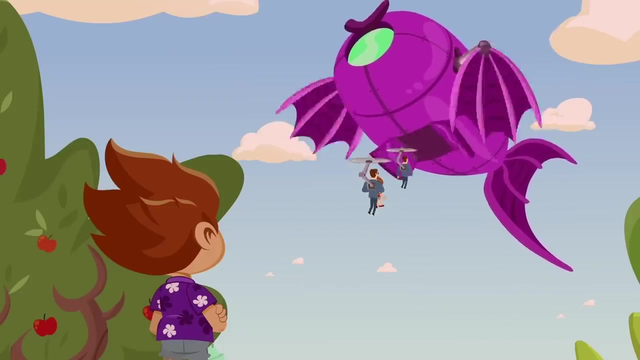 Of course, girls and boys. what happens with this magic mirror is that if we press the green button, a kind and good version comes out, But if we press the red one, an evil version comes out. How evil You're to blame for everything, Dr Spooky. 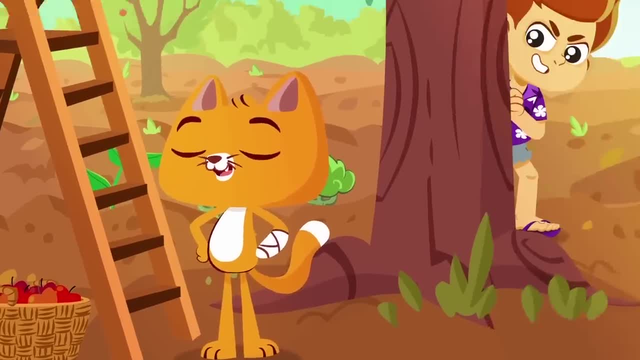 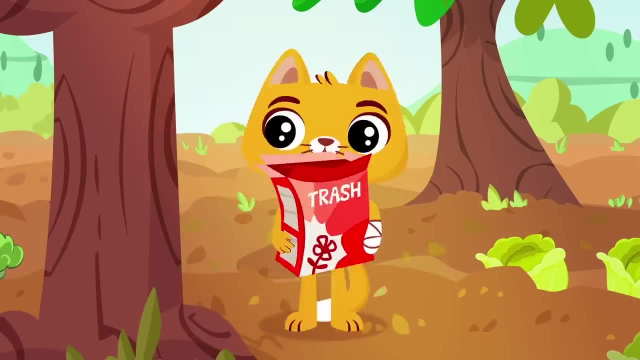 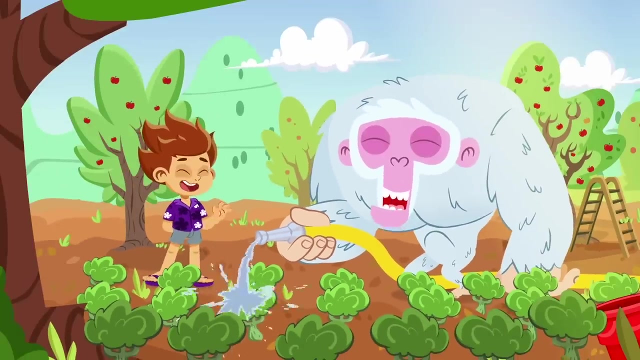 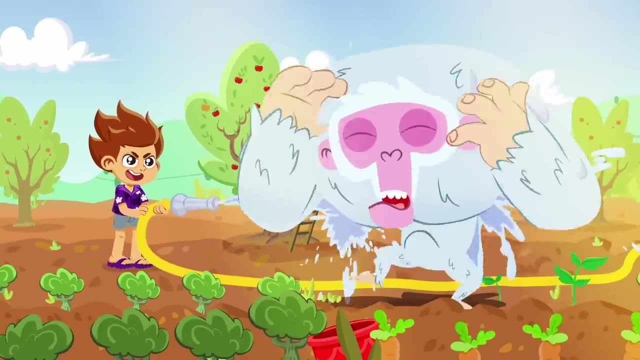 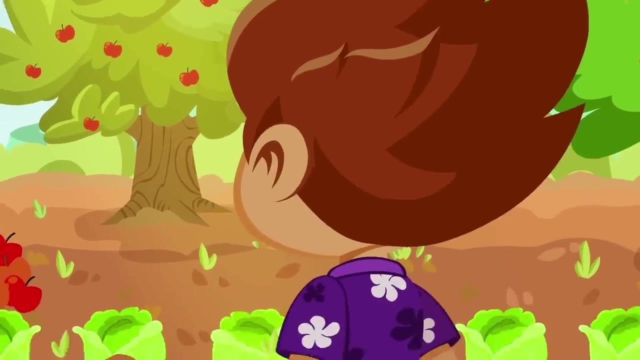 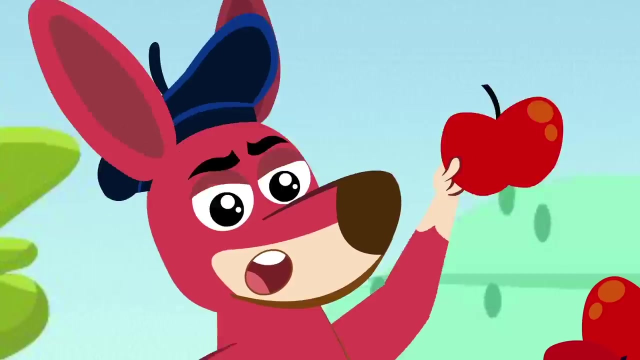 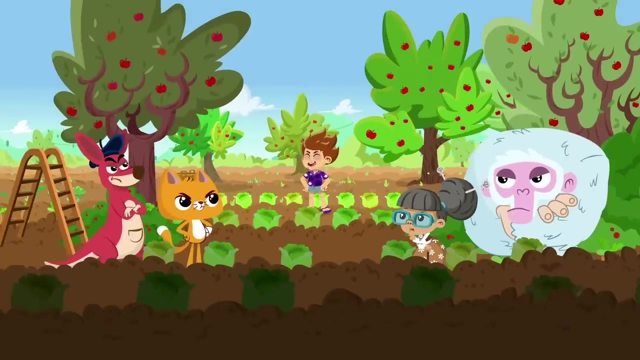 Easy kids. we'll help you. What's your plan now? Evil, Super evil. This is not the evil version of kids. This is the extra super evil version of kids. Granny, please, we have to do something, Hmm. 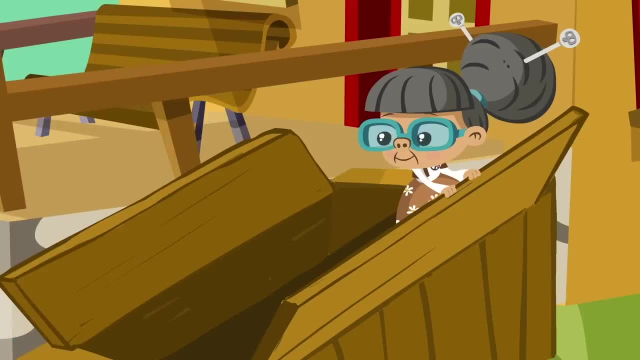 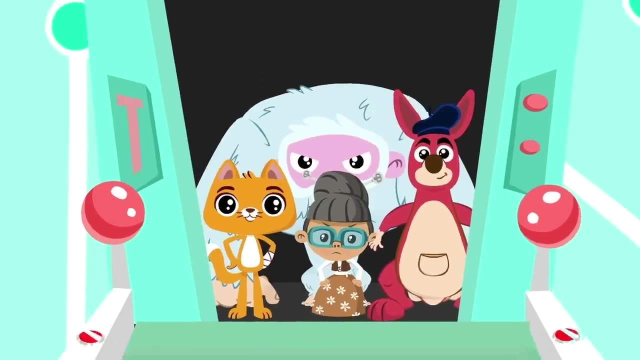 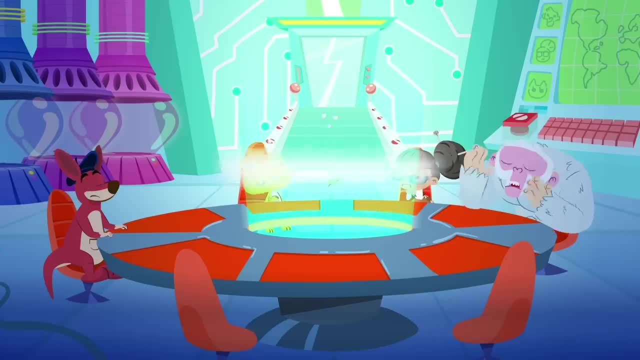 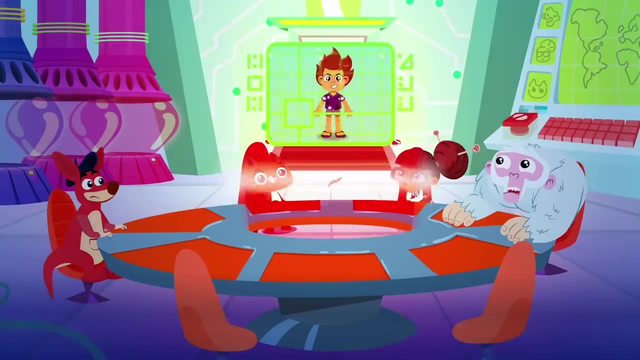 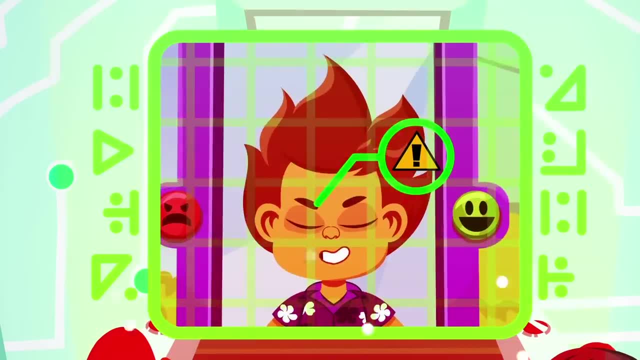 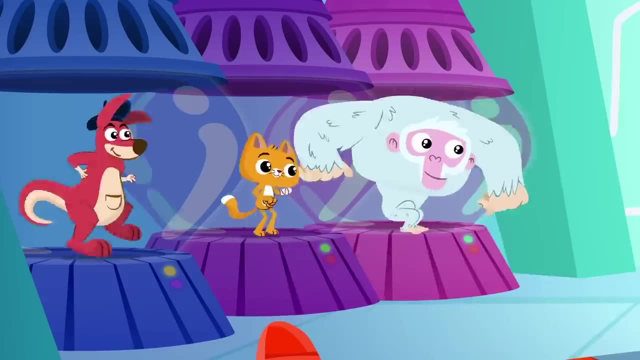 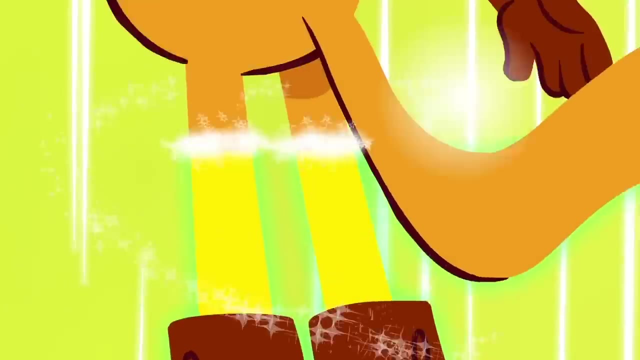 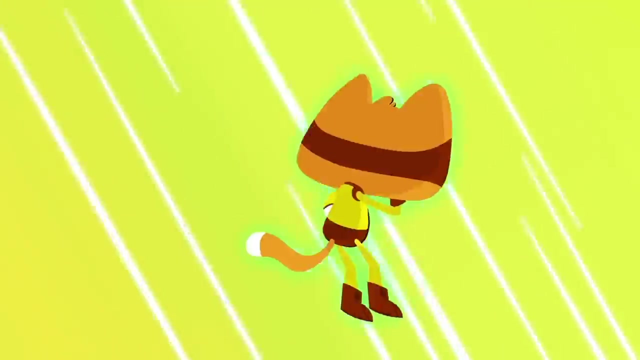 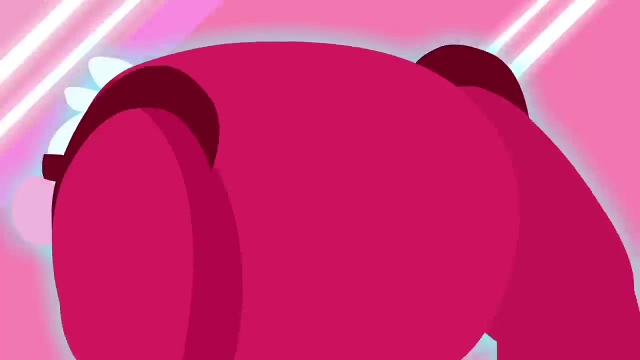 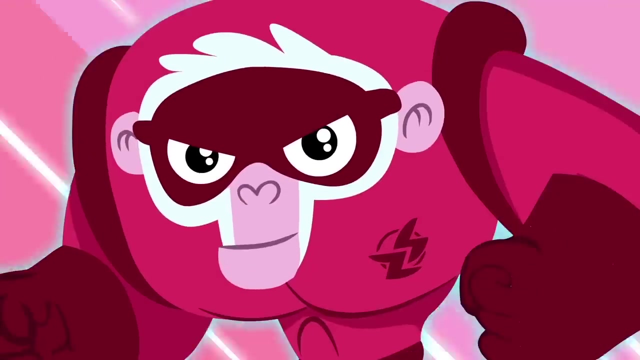 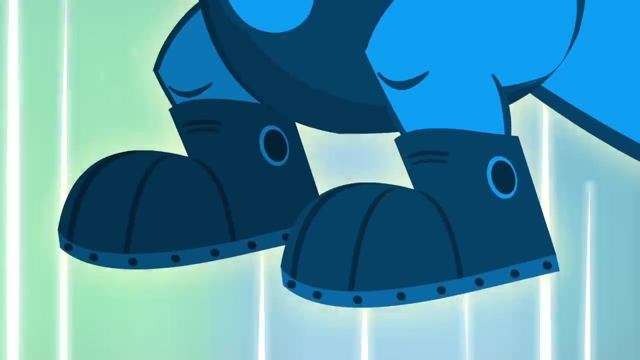 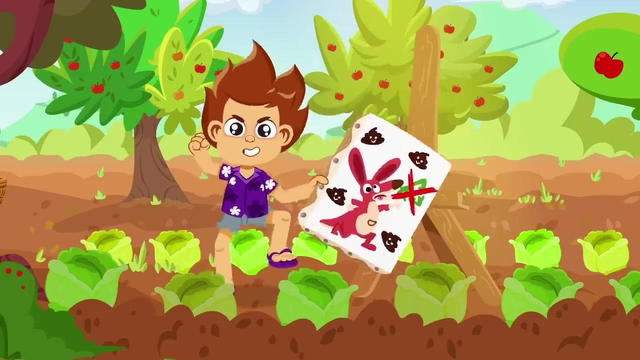 We have to stop the evil kid and save the REAL kid To the transformation capsule, Super Soup. Anyone watching, please like and subscribe my channel. Catty Monkey Canoe. Evil Kid doesn't seem to like Kangoo's art at all. 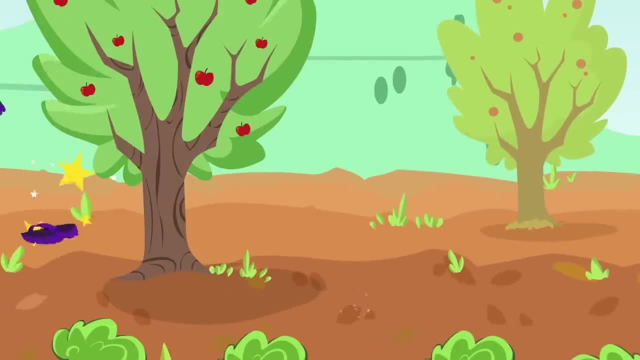 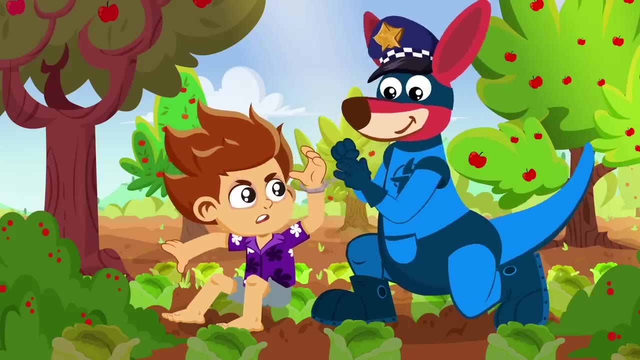 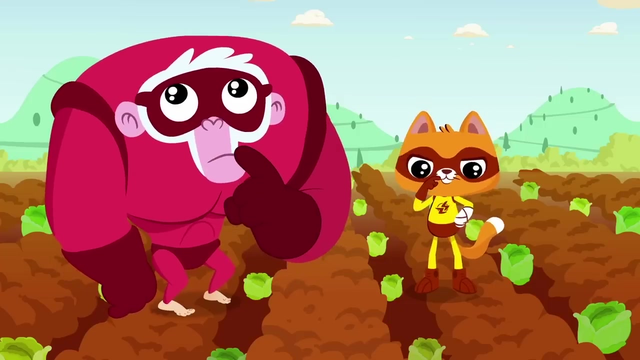 I'll admit it's a bit of a bad joke, but it was effective. Art Police, You are under arrest for being evil and having lousy taste. Sure Kid is probably on spooky ship, but he's not a ghost. But how can we get up there? 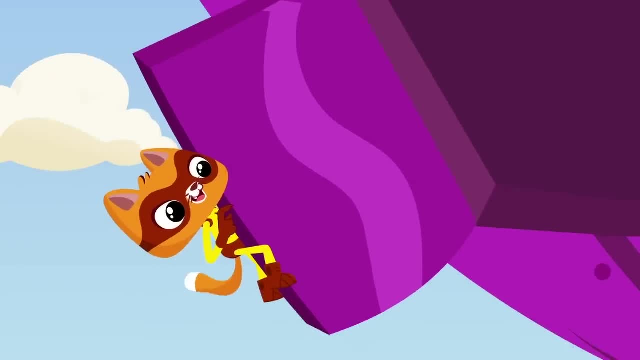 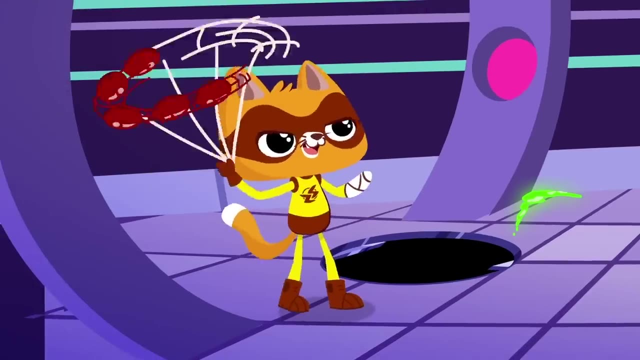 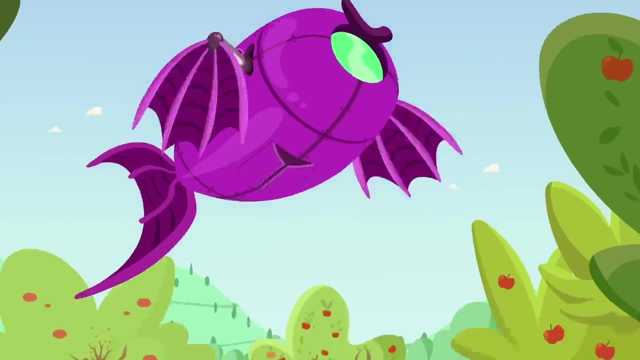 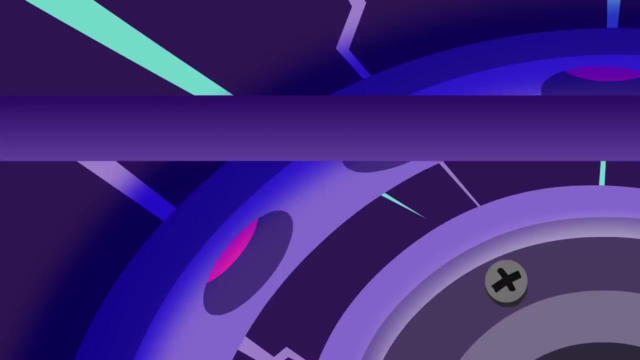 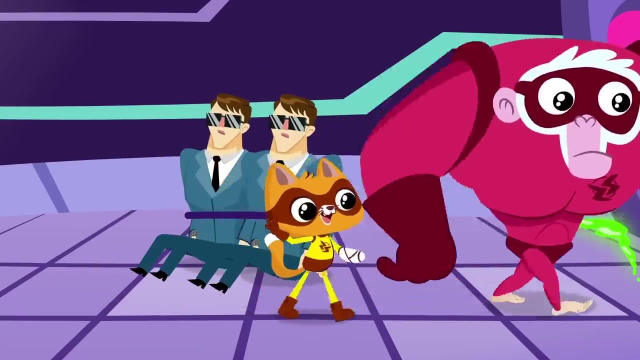 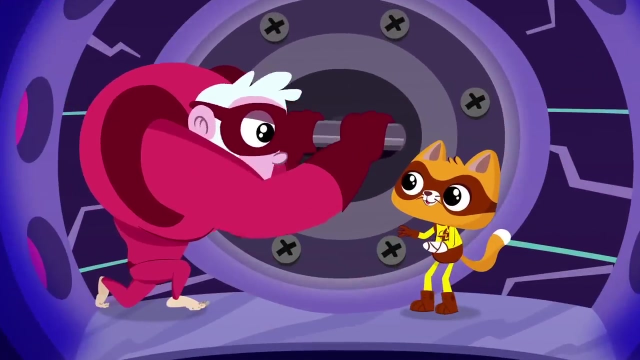 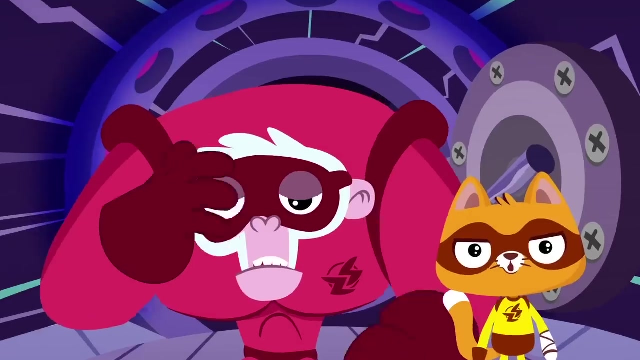 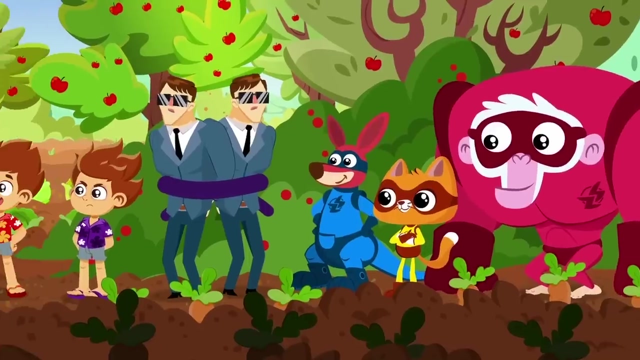 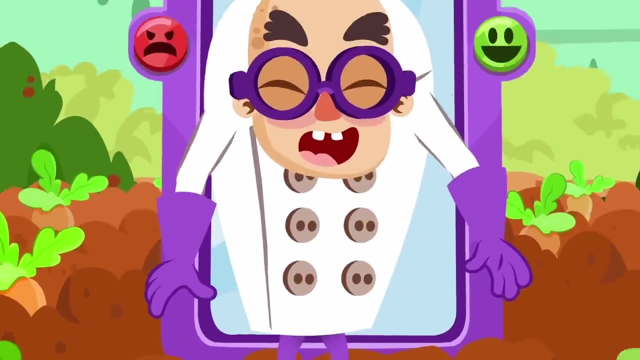 You're amazing, Perfect, Yeah, Hey Watch out. Wow, Amazing. Come on, We've got to find Kid. Will he be in here? Sorry to interrupt. We are here to save Kid. Huh, Uh, Oh, how cute. 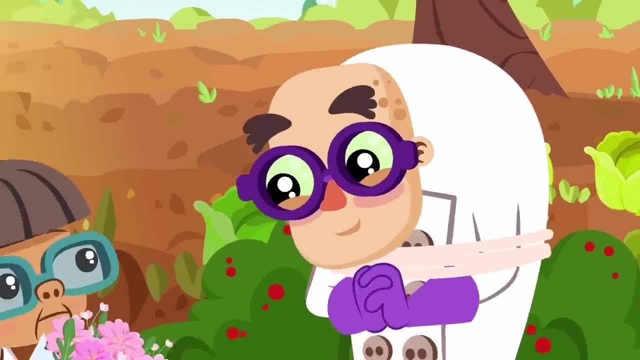 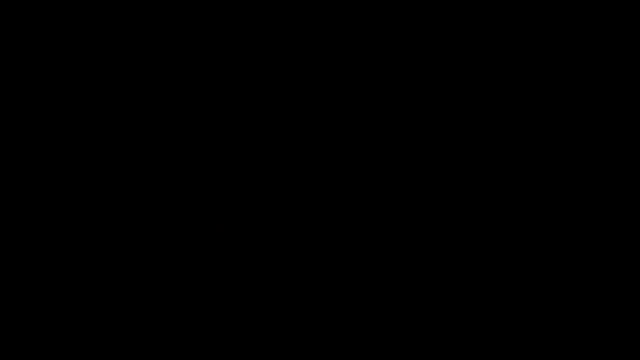 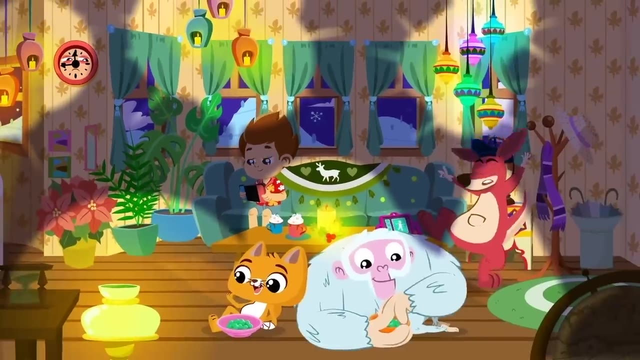 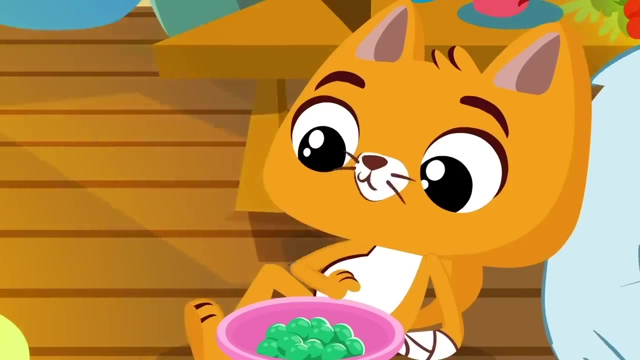 And remember we can all have a bad side. The important thing is to cultivate our good deeds, and that way we'll get lots of friends. Hello SuperSuit team. Isn't it too late for video games? Isn't it too late for snacking? 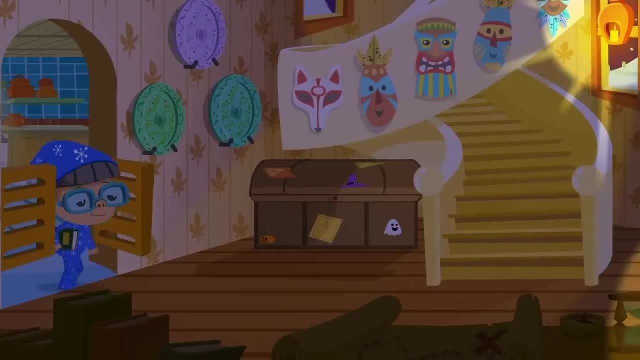 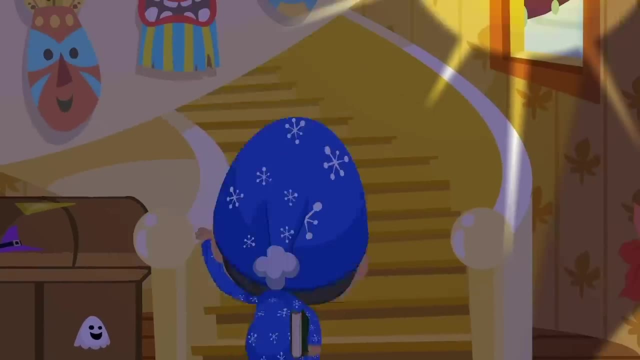 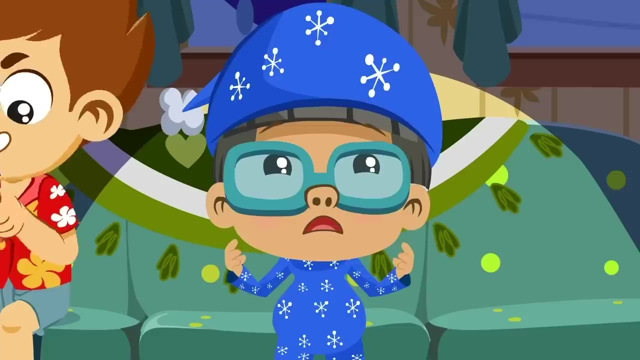 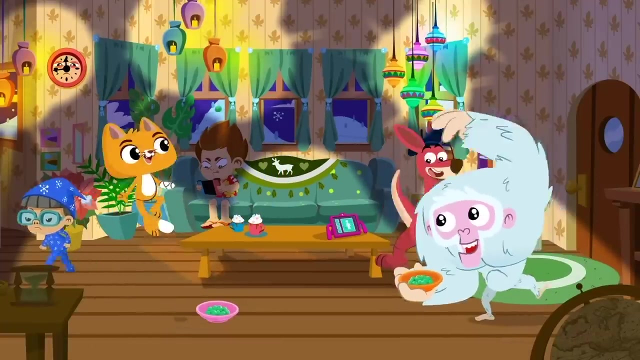 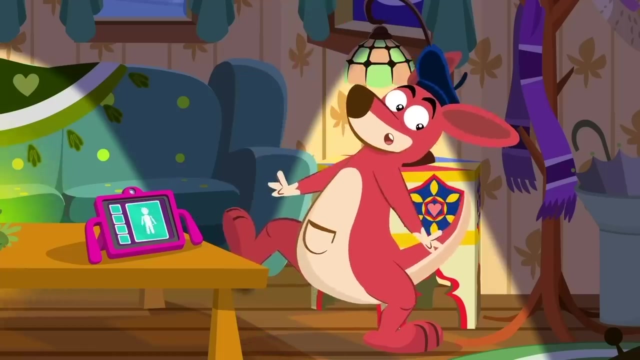 Isn't it late for dancing? Finally, Someone who looks like they're going to bed. I'm as shocked as you are. They can't hear you. Granny, It's already too late. Granny's right, You have to go to bed. 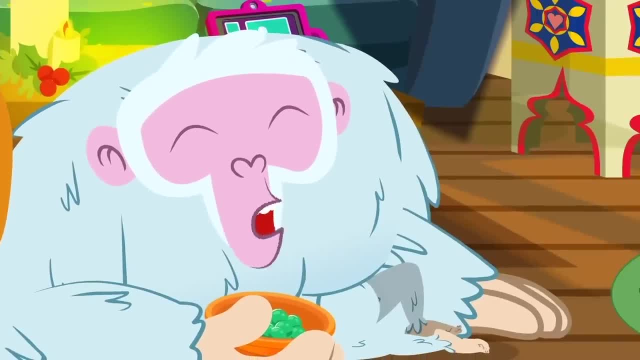 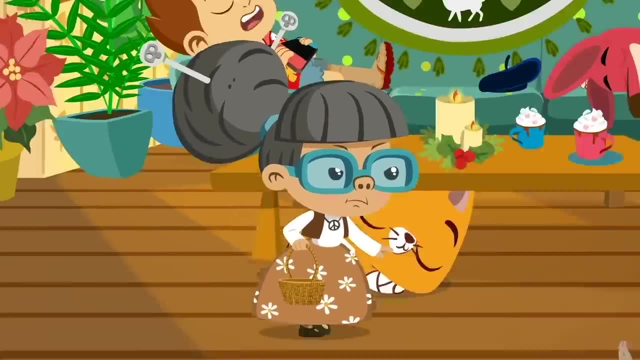 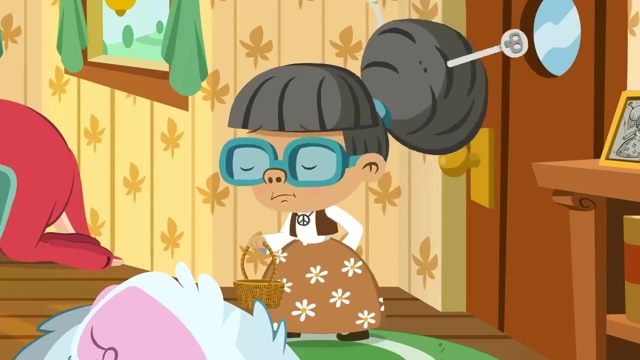 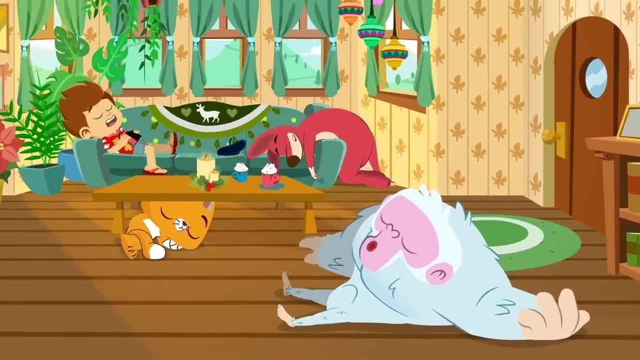 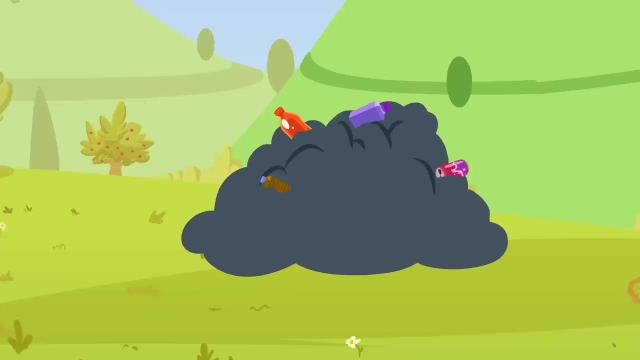 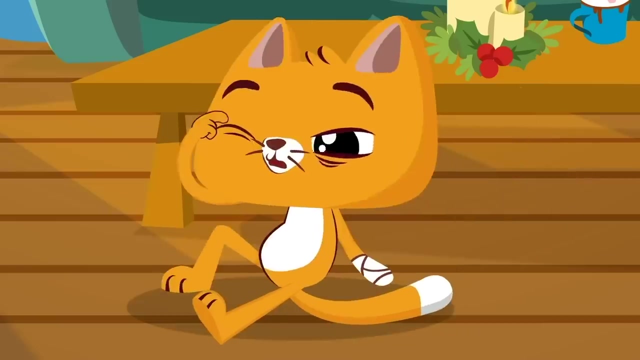 Come on, Go to bed. Alright, Do what you want. Good morning, I said. good morning, Oh Lord. What? What's going on? Oh, no, Evil. Dr Spooky is filling everything with garbage. Where's the SuperSuit team? 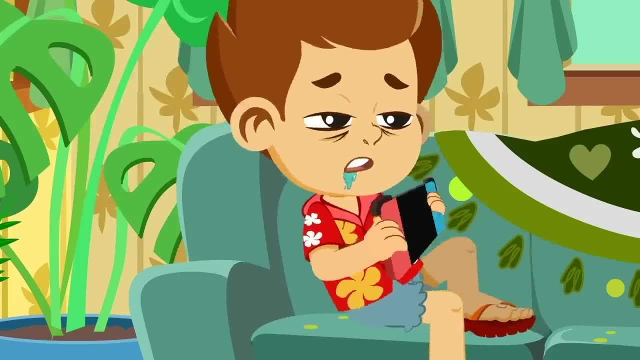 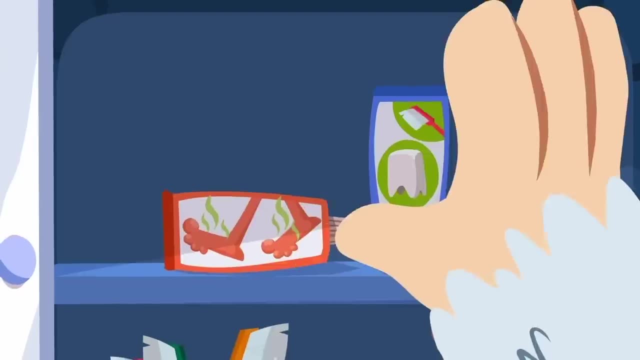 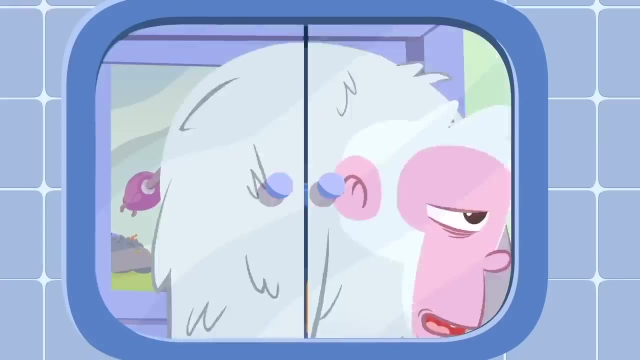 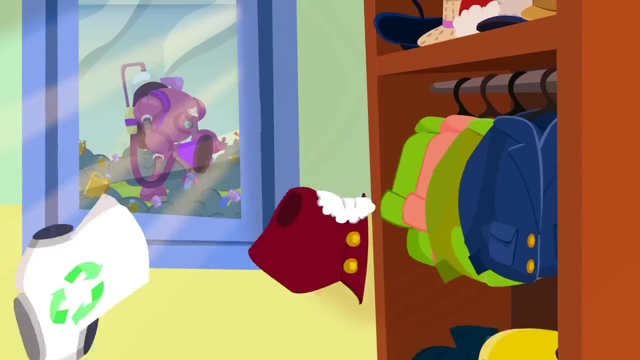 Huh, Oh Heyo, You guys are finally on the move. Thank you, Uh-oh, This is what happens when you don't sleep well. I have no idea what they're doing either. Spooky. This is what happens when you don't sleep well. 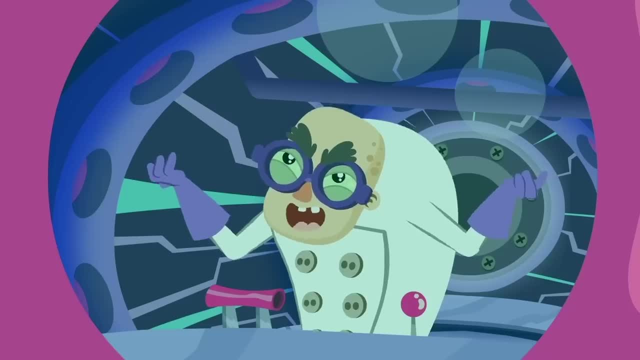 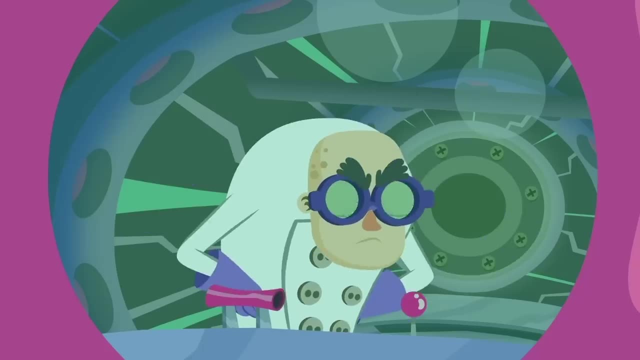 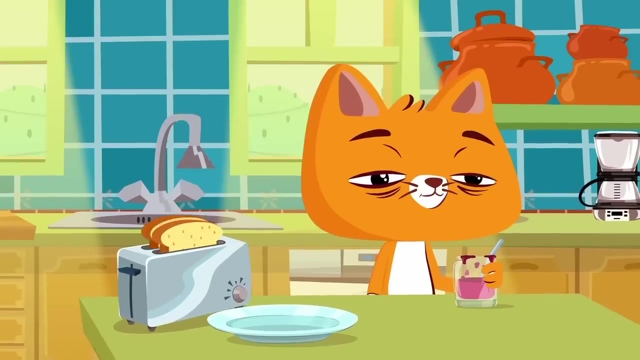 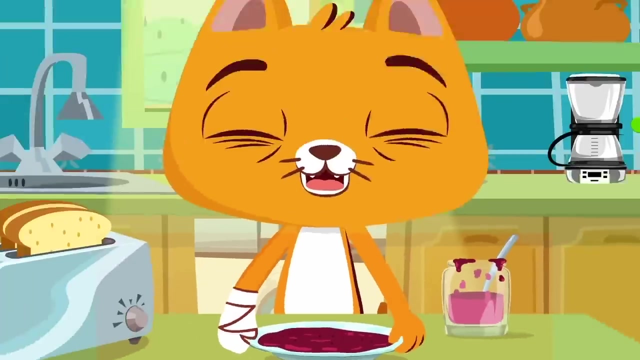 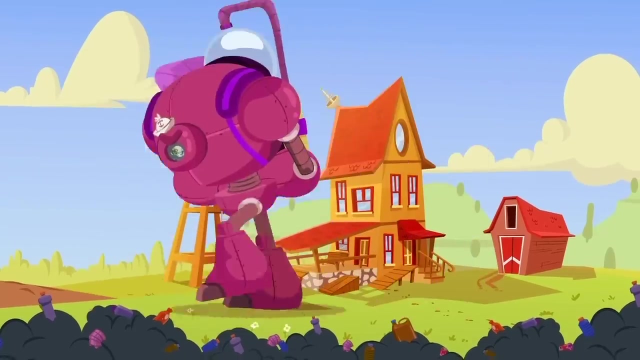 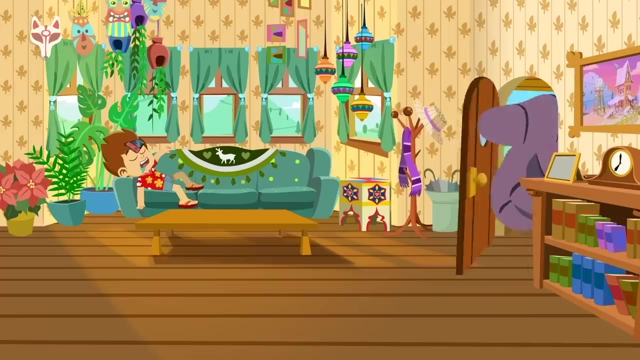 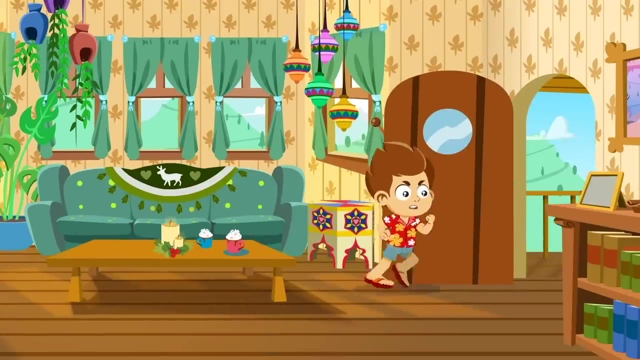 Spooky is making a huge mess. Is this a joke? Team SuperSuit, let's go. Here's Catty. This is what happens when you don't sleep. well, Hello, It's time to save the world. Um yeah, This all happened when you were asleep. 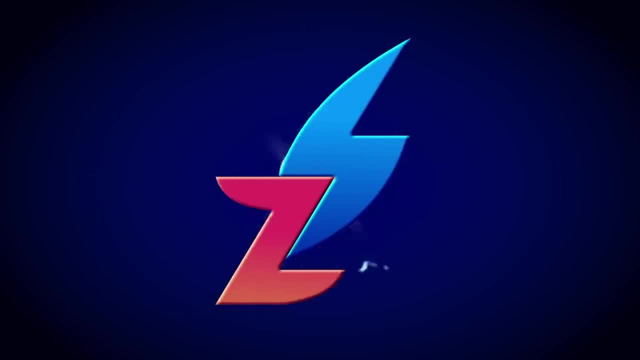 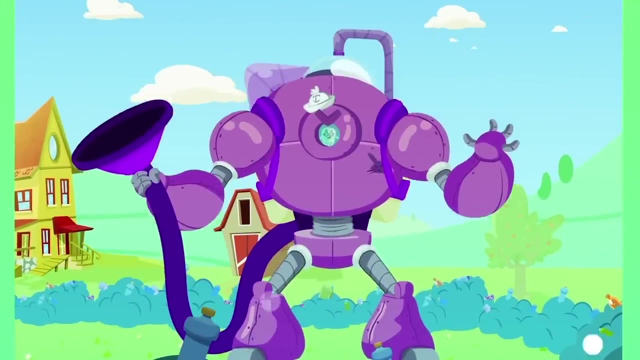 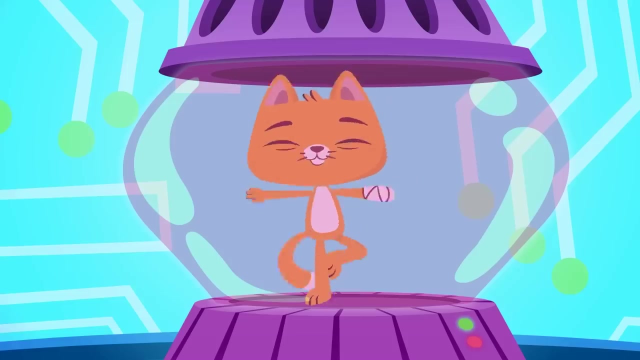 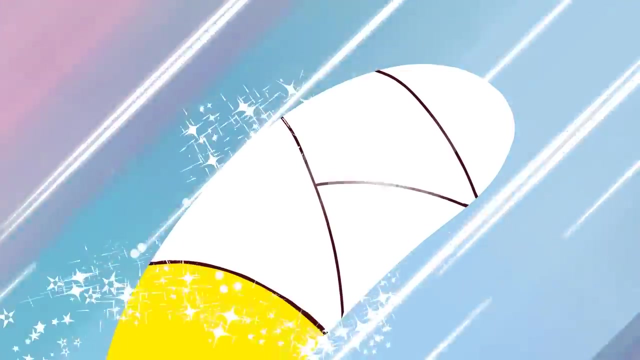 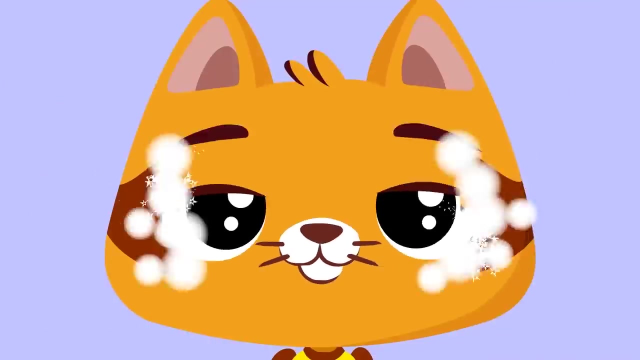 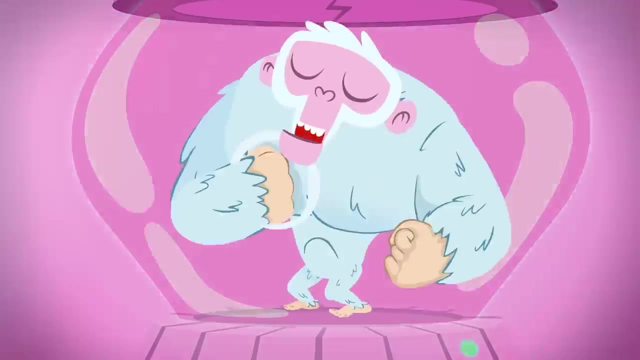 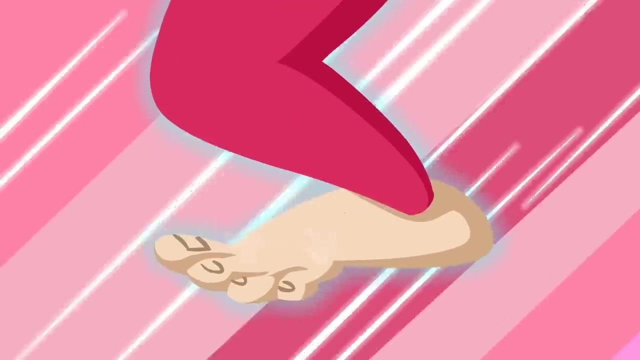 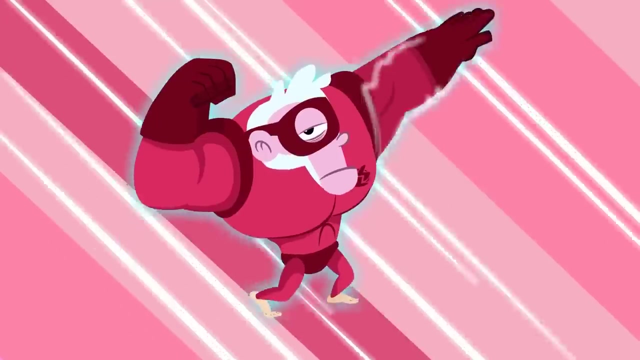 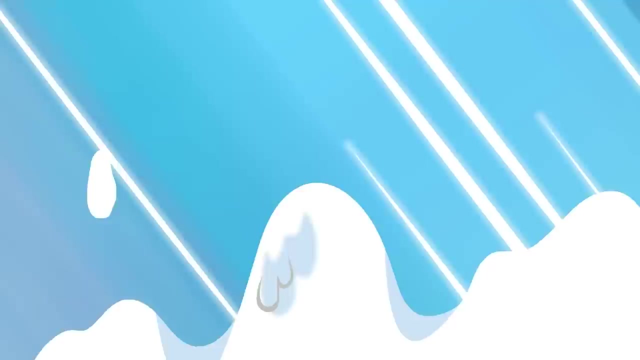 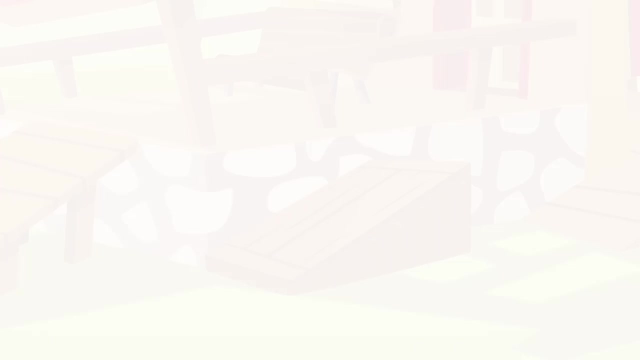 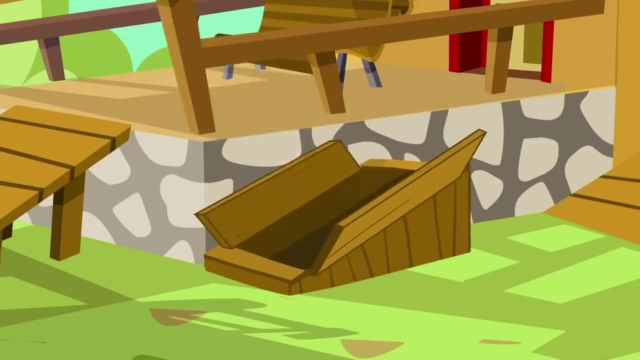 We had to stop the robots and clean the field. Knock, knock, Get your act together, guys. we've got to stop Spooky to the transformation capsules. Let's go Spooky. Let's defeat Dr Spooky once more. 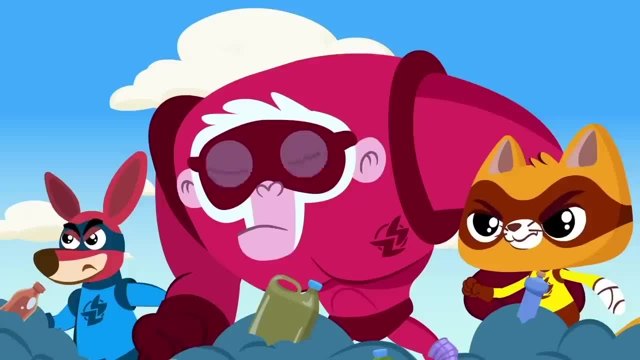 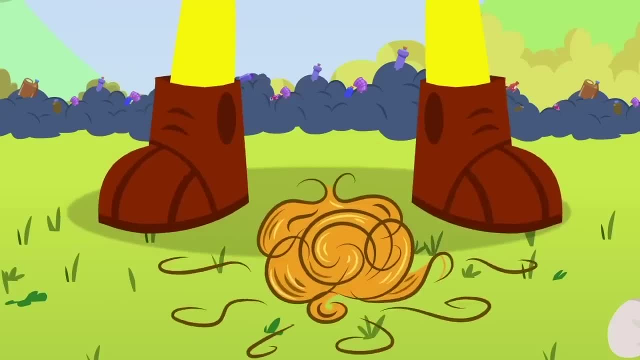 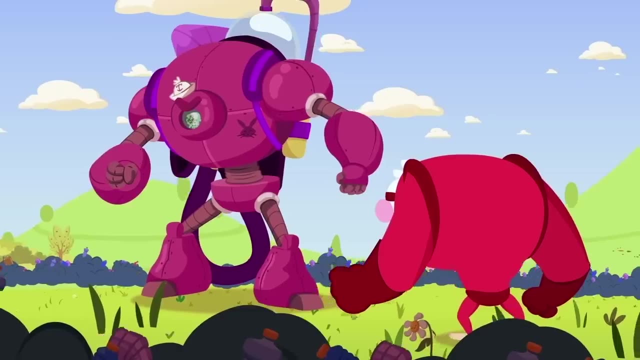 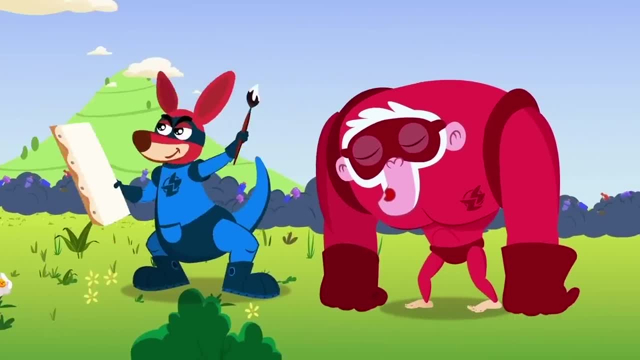 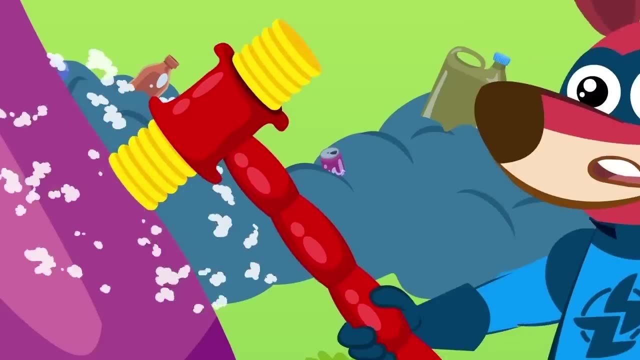 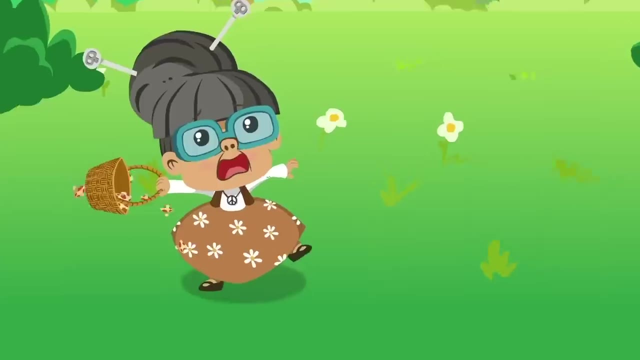 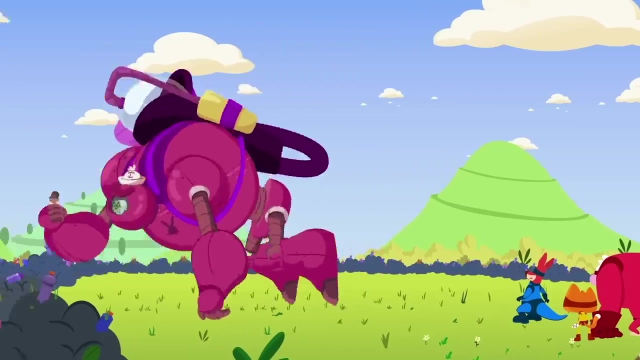 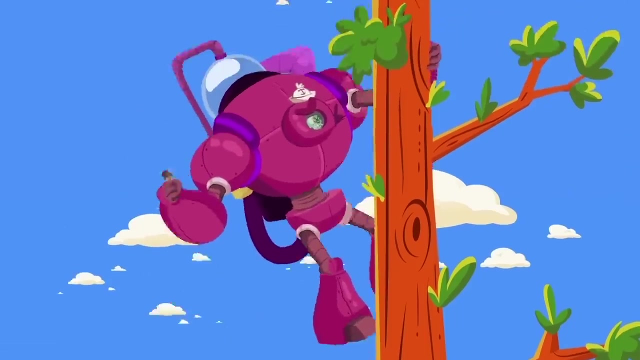 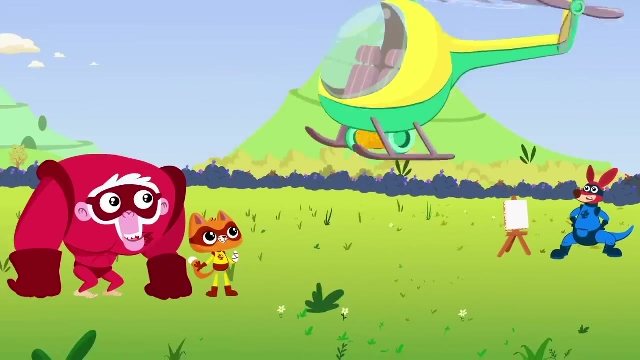 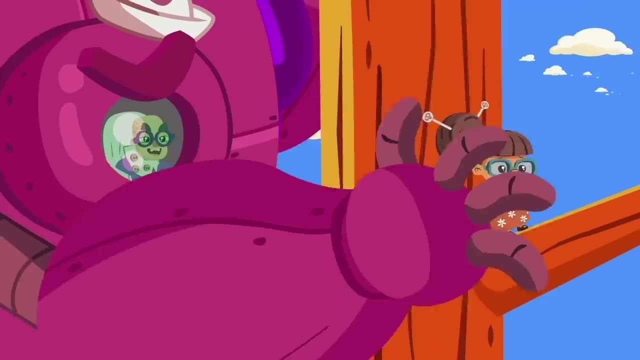 Spooky No Monkey. Come on, Kangoo. Today everything goes wrong. Watch out Granny. Go Super Suits Team. It's taking Granny away. Do something, esse. How cool, Great. Now let's all show the power of Team Super Sue. 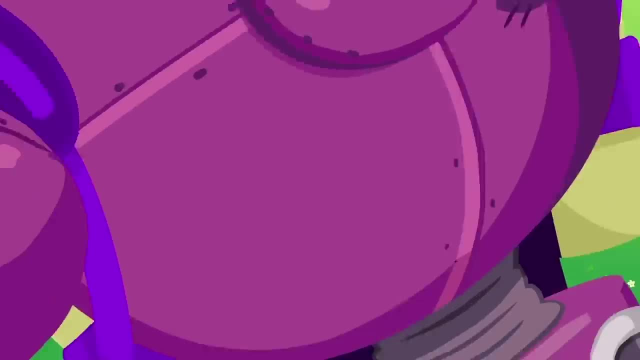 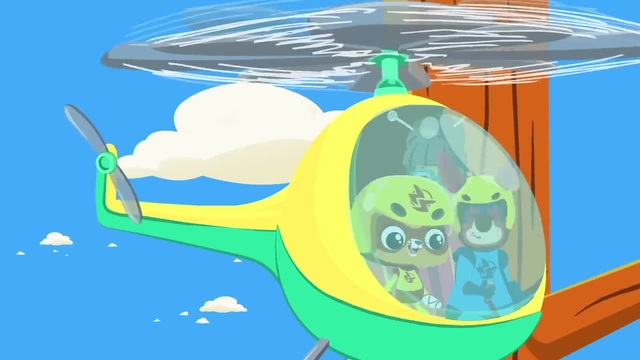 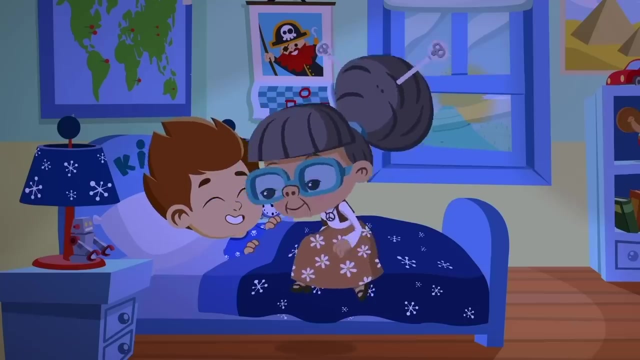 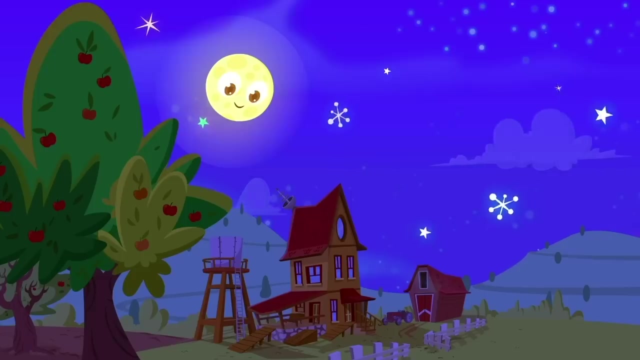 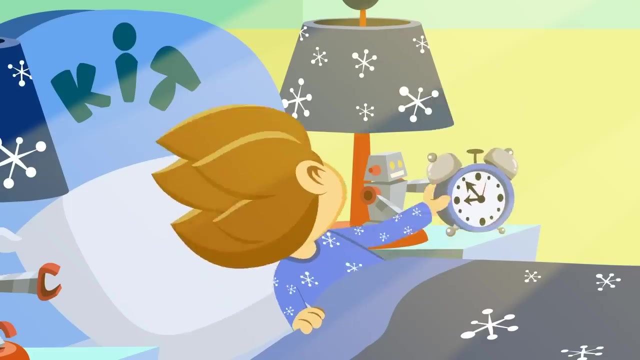 Right on target. Bye, You're the best And you're a great team. Go to sleep And remember kids. If you don't want your day turned upside down, you've got to get into bed early. Sweet dreams What. 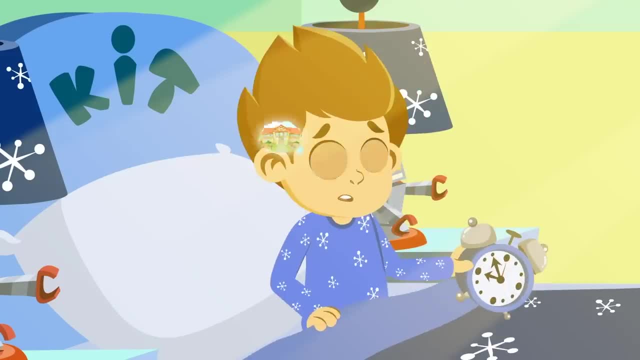 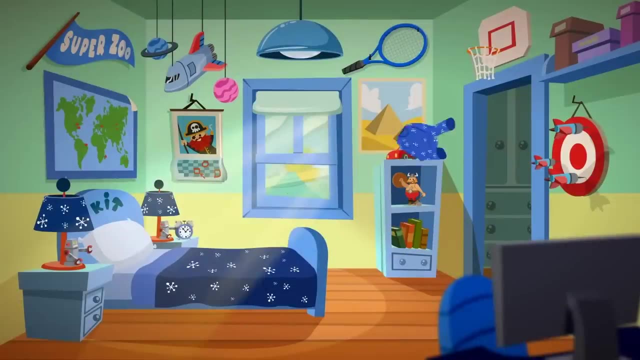 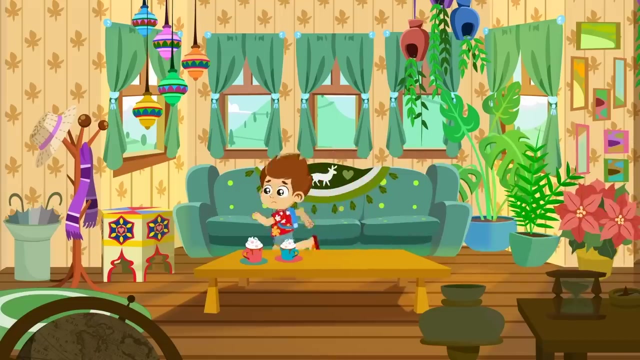 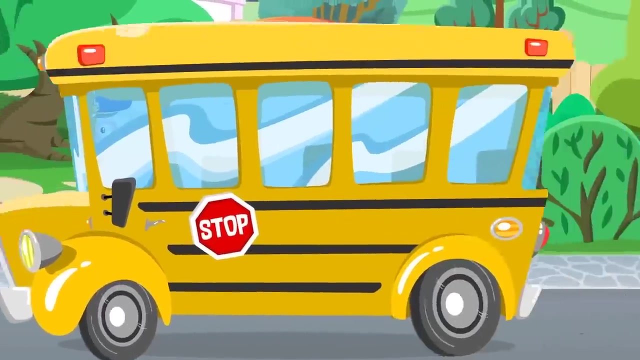 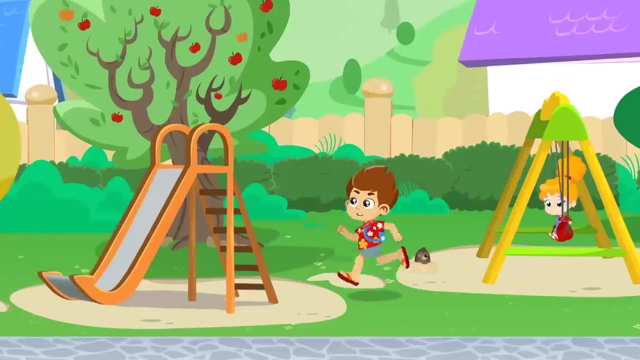 Five to nine: Kit starts school at nine. Oh gosh, he's going to be late. There's no time to lose. Let's go, Kit. Get your backpack and your books. There's the bus Faster, Kit. Let's go, Kit. 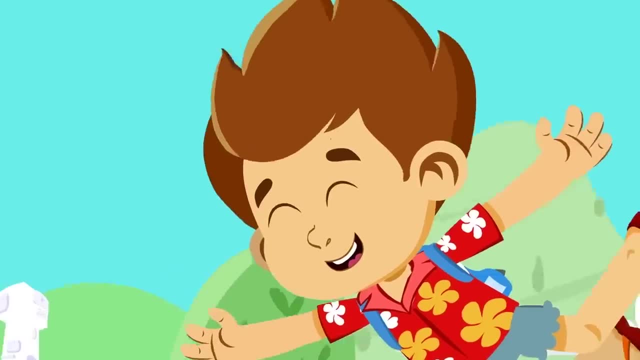 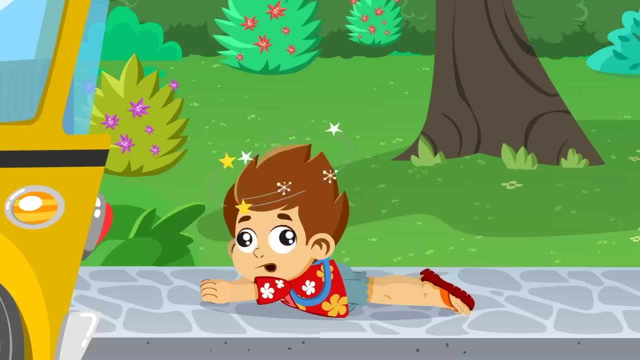 Where is it? Here it is. This is the bus, Don't worry, it's here. It's still waiting for us to get out of bed, But you'll have to wait a little bit longer. Hey Kit, Why don't you pay the bus? 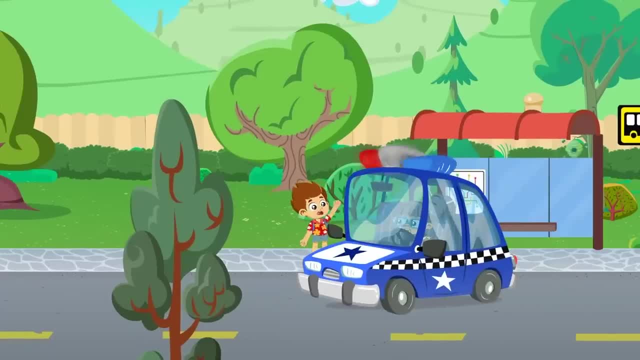 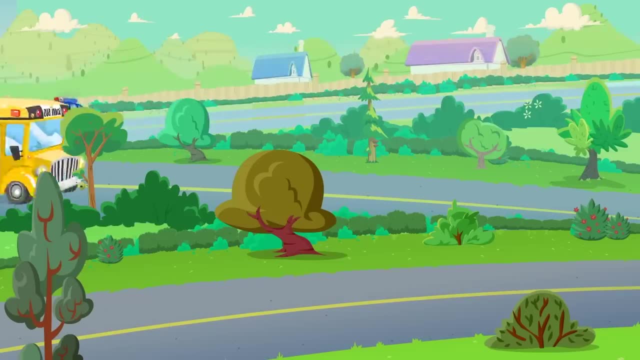 No, My driver is in trouble. Hey, I have a question for you. What is it? What is it, Kit? What's the matter? I'm late. What's your problem? Don't worry, I'm not late, I'm late. 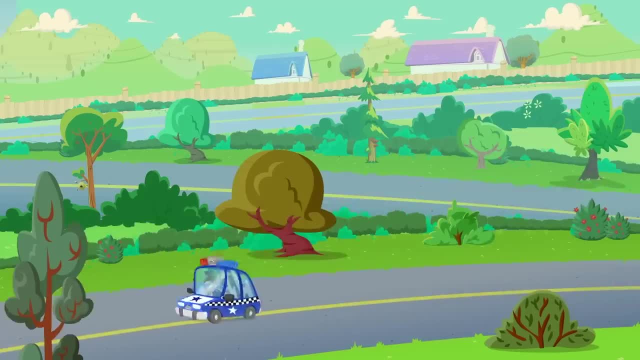 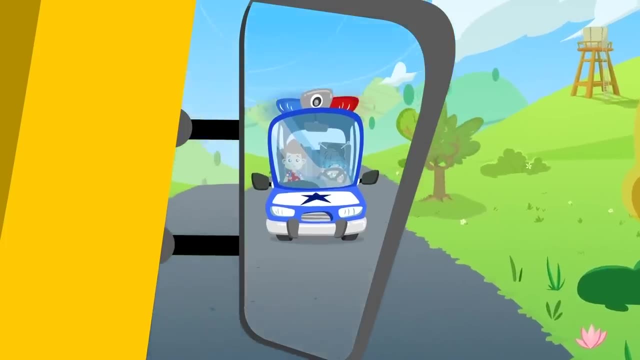 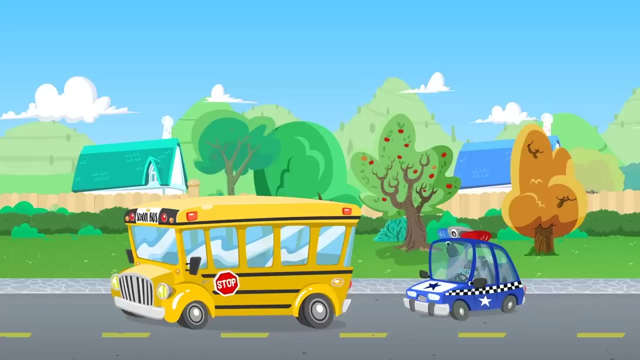 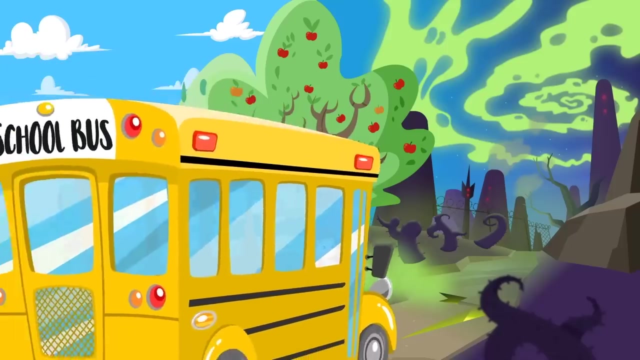 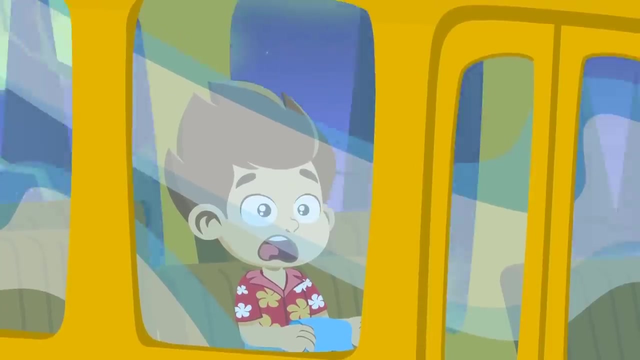 Hey, it's Monkey and Raccoon Guys, stop the bus, Finally, Phew Kit will make it to school on time. Um, are you sure it's this way, kids? Uh-oh, we've entered evil Dr Spooky's compound. 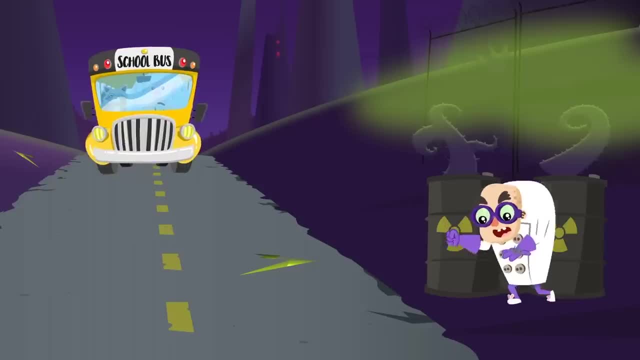 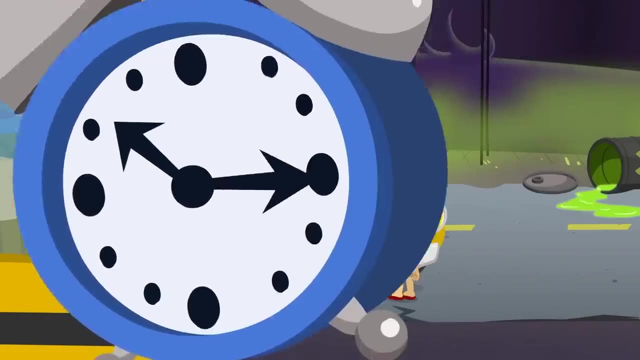 I told you there's that scoundrel And he's thrown some spikes onto the road. One of the tires blew out. Oh, and where are we now? We need a stroke of good luck, And that stroke's name is Patty. 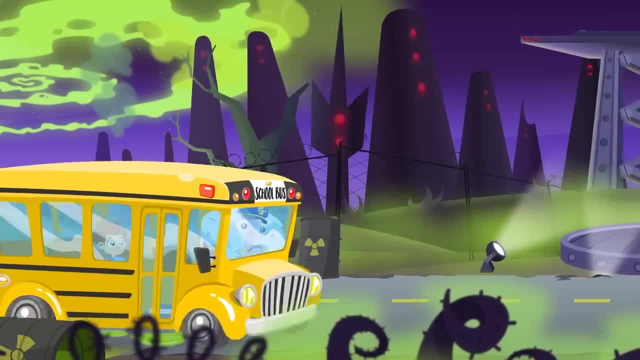 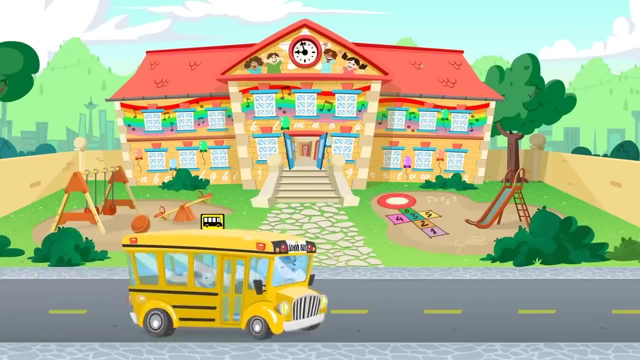 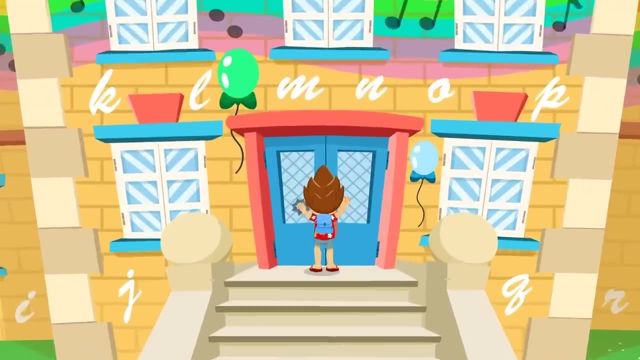 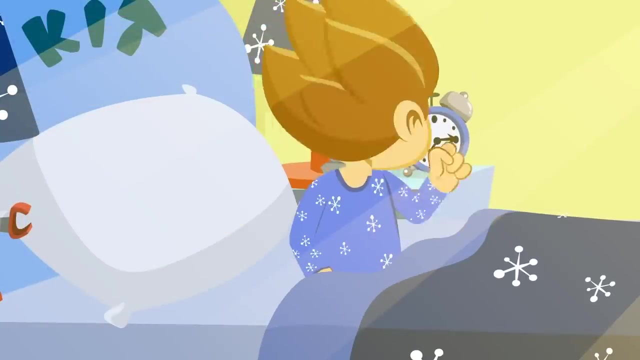 Express Roadside Assistance Service. Let's keep going. We're almost to the school. Run Kit. Oh no, He didn't get there on time. What? Of course, It was all a dream. It's 7.15!. There's still plenty of time before the school opens. 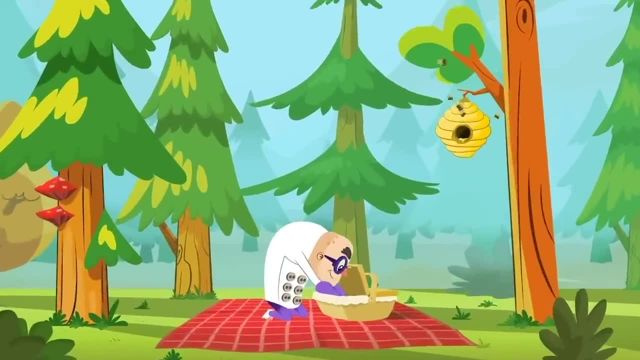 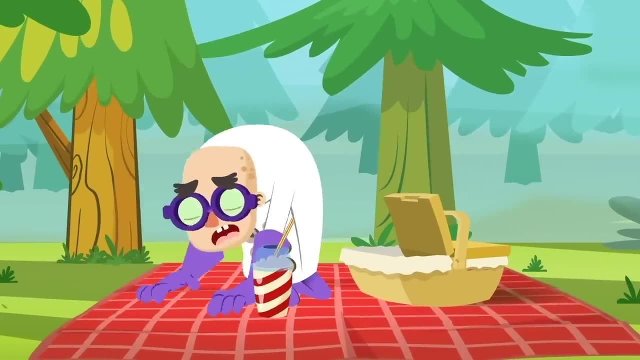 What a relief Kit. Dr Spooky is having a picnic. He's going to eat a greasy hamburger. Oops, guess not. How about that milkshake? Nope, not that either. Will he be able to eat the ice cream? 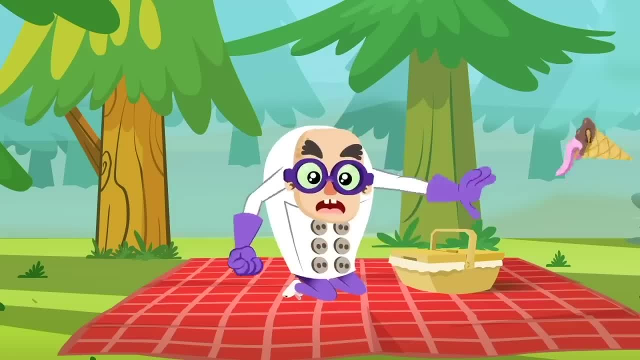 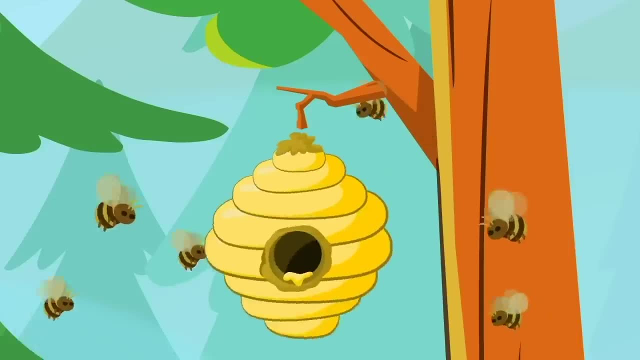 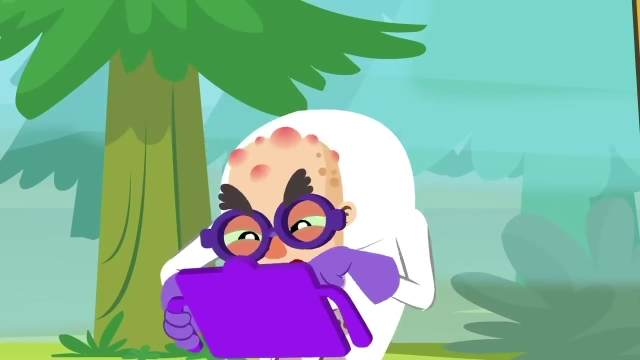 Haha, In your dreams. Wow, Dr Spooky doesn't like nature at all, And nature doesn't like Dr Spooky at all either. Oh no, What's this? What's this? Why is he summoning his robot? 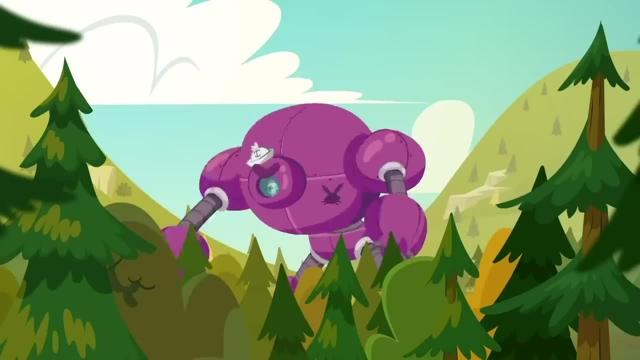 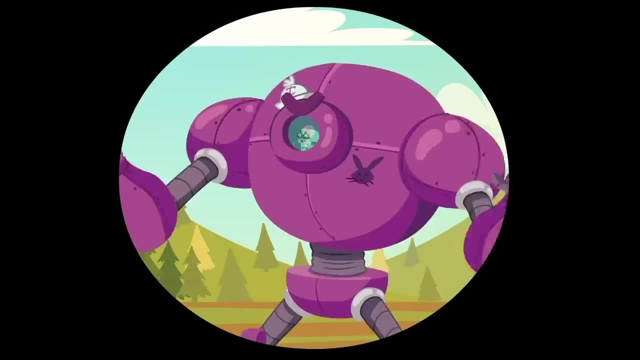 Look at that, watch out. Wait a minute. Dr Spooky is uprooting all the trees in the forest with his robot. Yes, Granny, Just as you can see Dr Spooky's up to his shenanigans again. 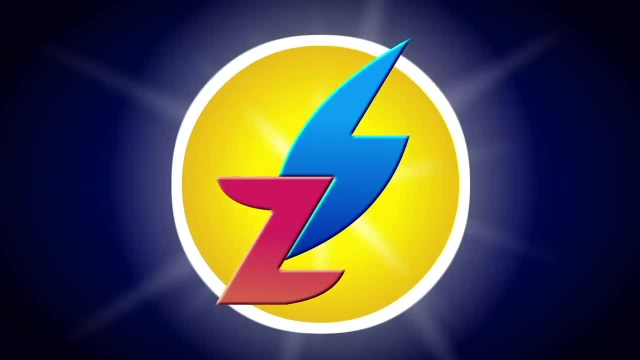 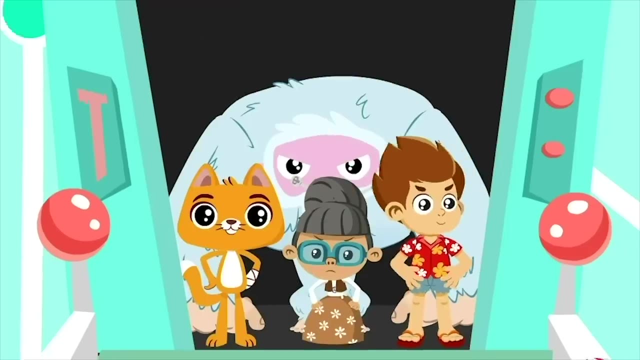 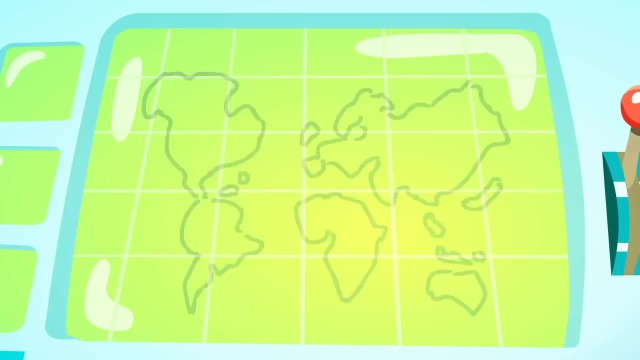 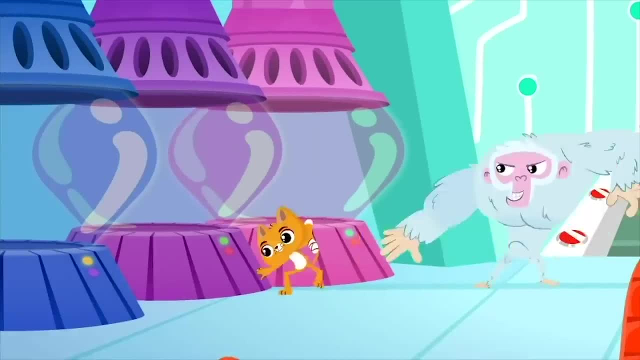 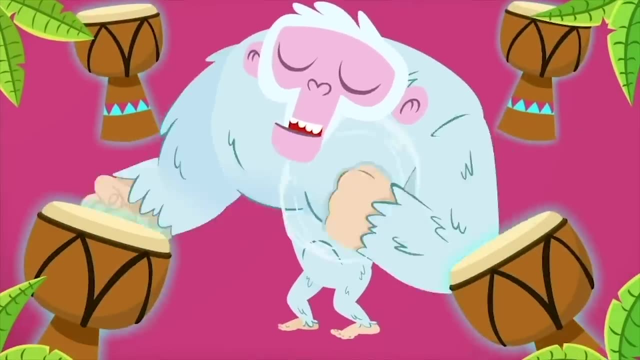 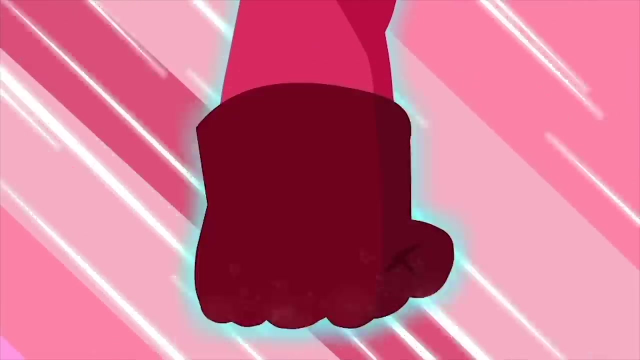 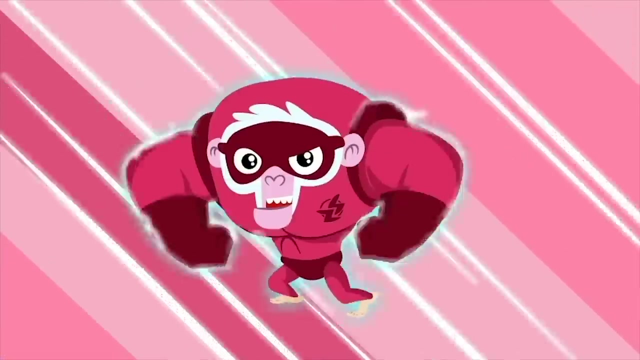 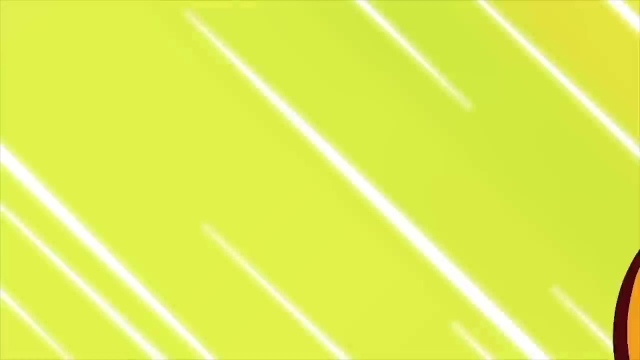 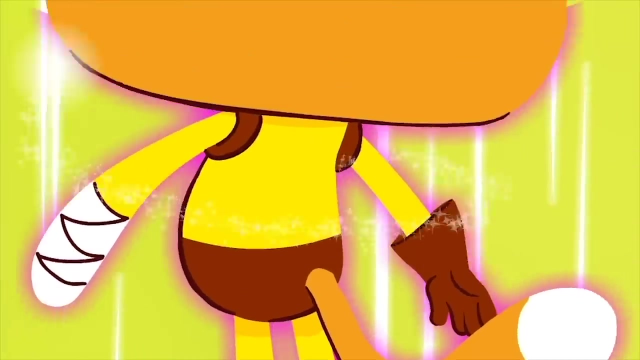 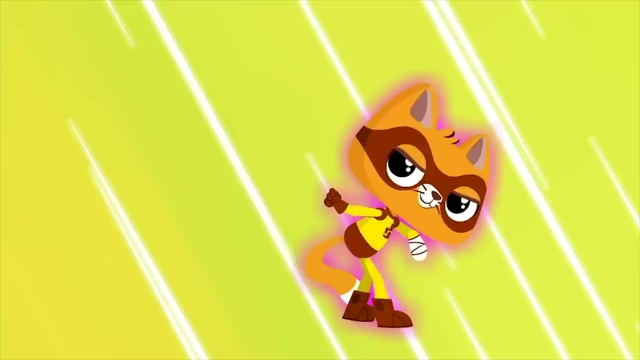 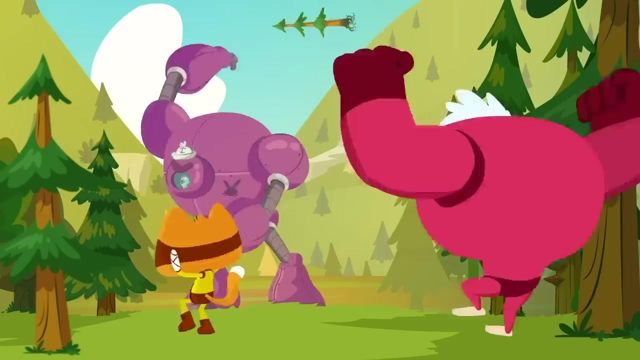 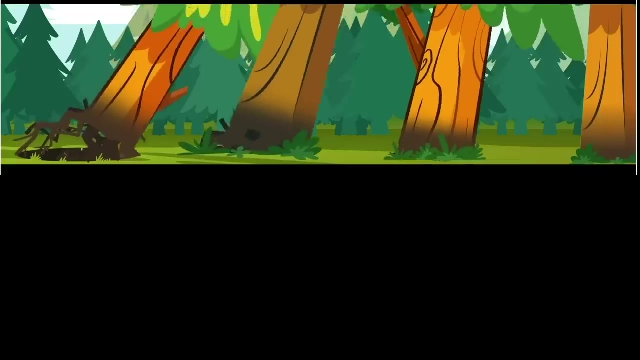 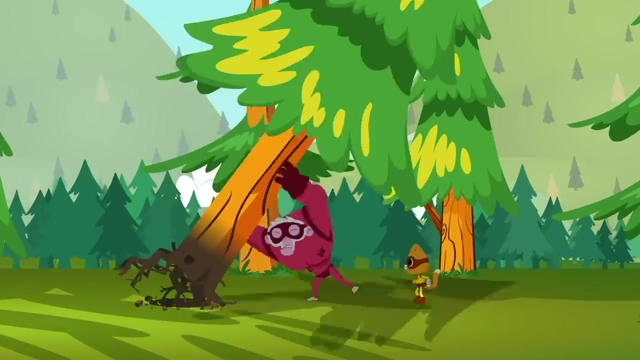 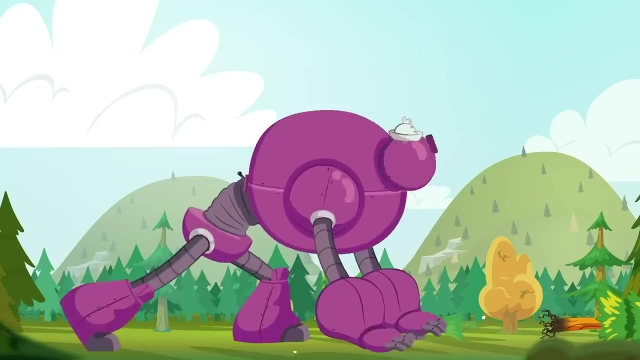 to control the robot, To the transformation capsules. Hmm, Monkey Catty, There's Dr Spooky, Watch out. No, What Wait? a second Great Monkey has stopped the trees. Now we're going to protect the environment. 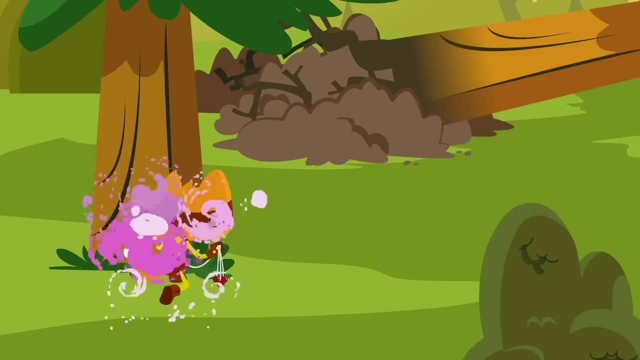 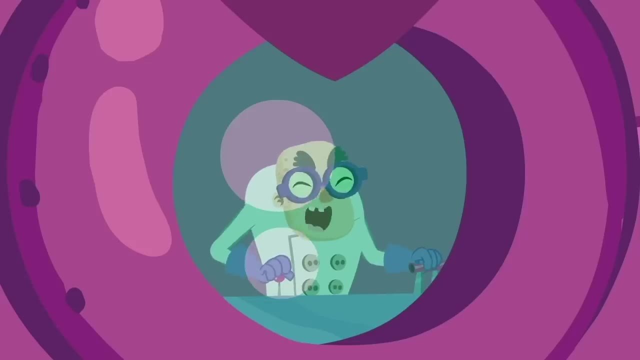 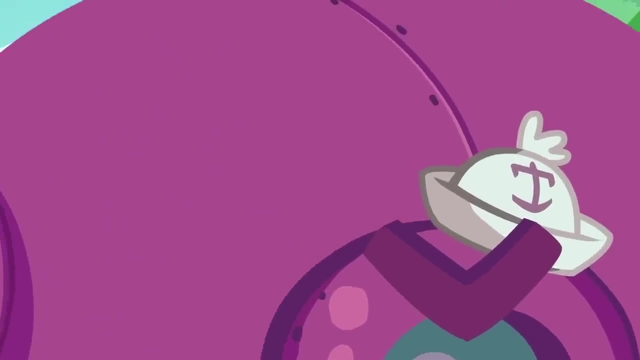 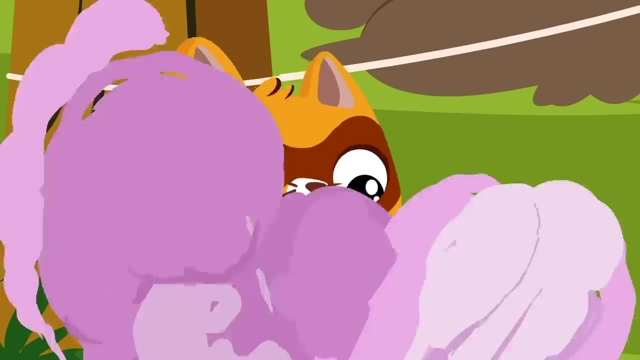 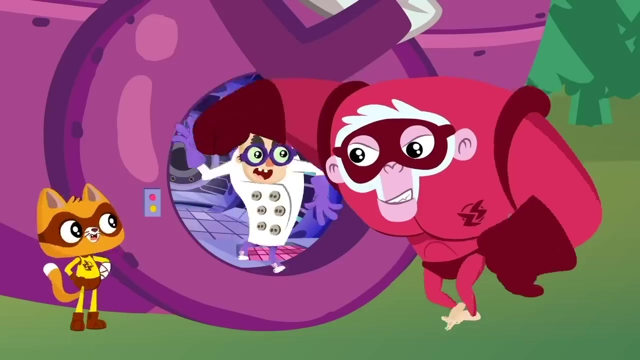 Uh-oh, Nice aim, Catty. See you later, Dr Spooky. Great job, Catty, You're the best. Now what, Dr Spooky? There's the button. Don't let him get away. Good wave. 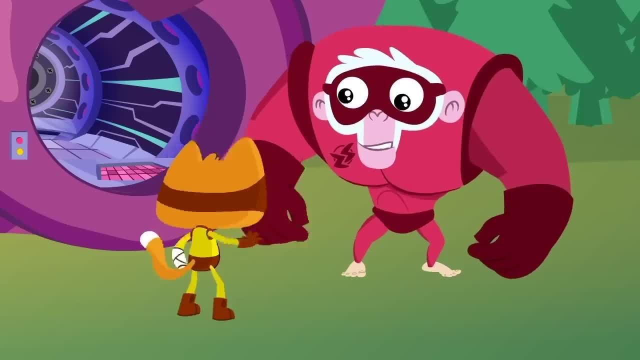 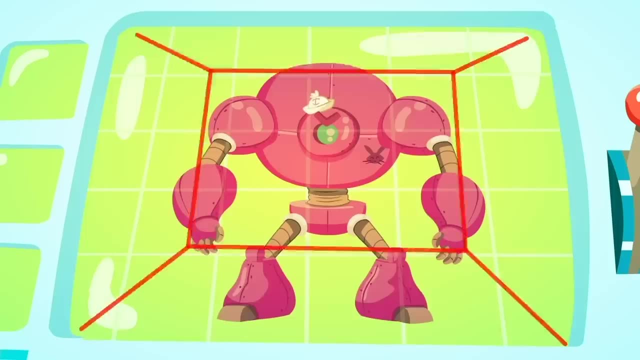 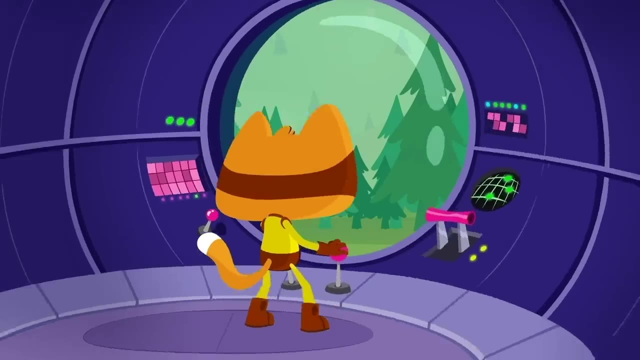 Aha, Gotcha, Uh-oh, Go. Come on, Catty. It's time to bring the forest back to life. We have to replant. Get up, Mr Robot. We have to fix what Dr Spooky messed up. 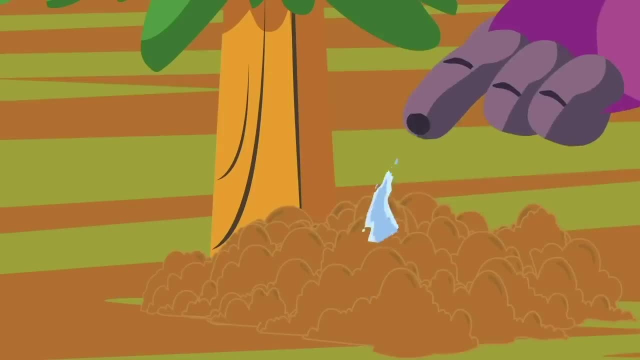 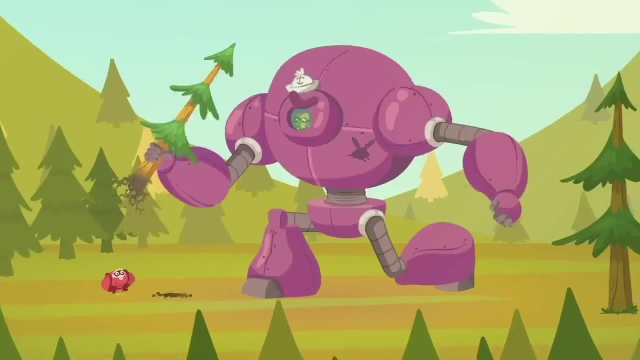 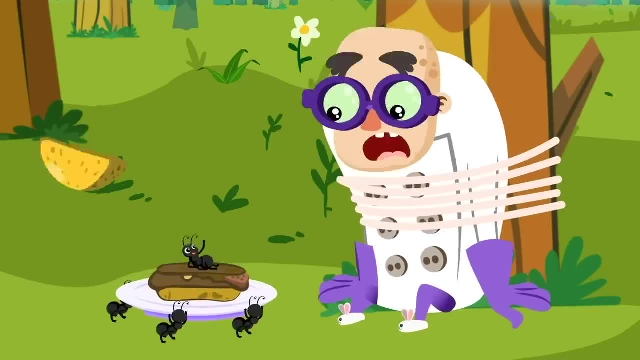 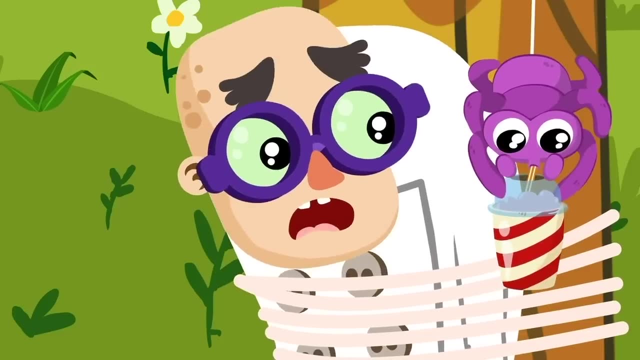